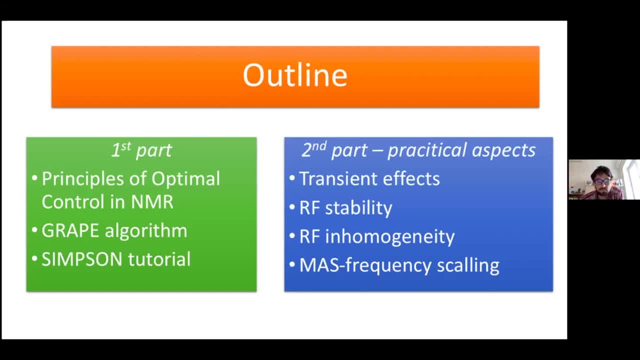 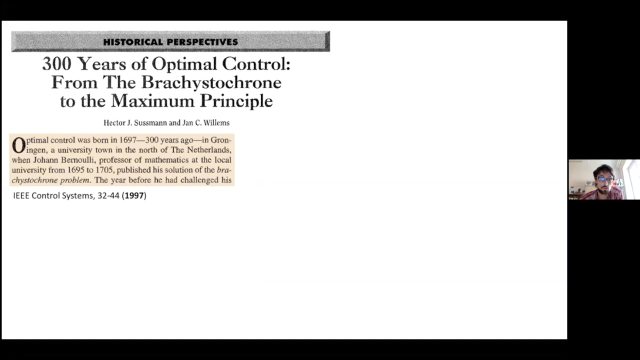 optimal control application with different troubles to be overcome, like transient effects, RF stability, RF homogeneity and also some mass scaling and reproducibility of optimal control sequences. So, without further waiting, let's go ahead. Optimal control is the group of tools or 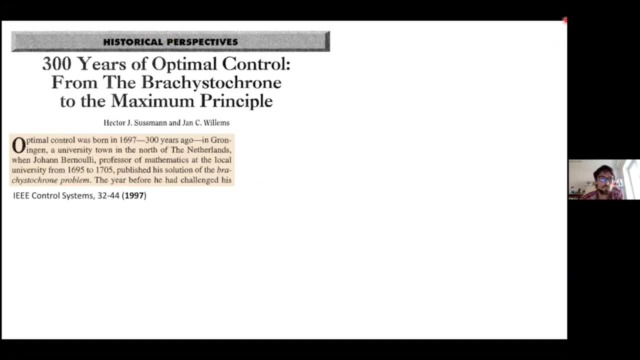 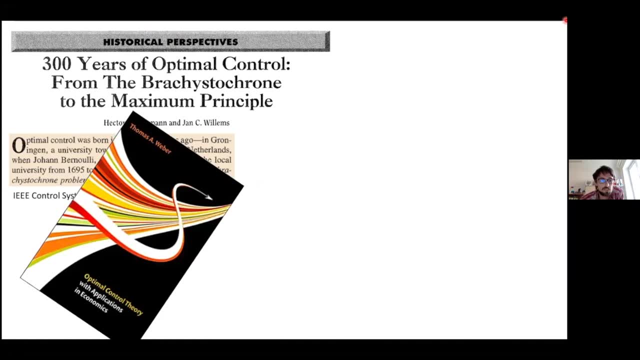 a bunch of tools which was just known for quite a long time. First sign was at least 300 years ago, But it founds its biggest application in economy in the optimization of the profit and resources. But it was also used, for example, by ISOM brother Bertko Zhori, a farmer in Rome in the 1952s as well. 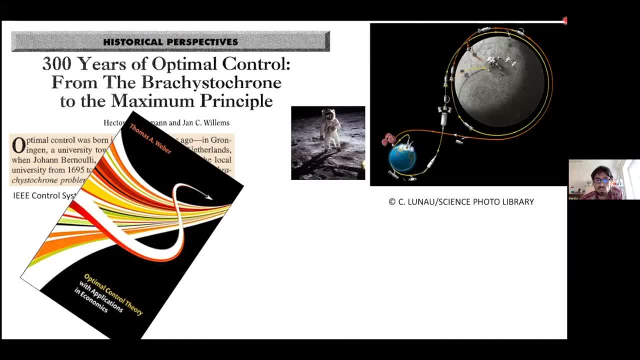 engineering 2D, new programming that spores much, millions of points, creating practical and환ormous tactics and easier solutions for optimal control and quality too. For example, it's generally used in the, for example, in the control of the spacecraft, in the economy of fuel during the, during the Apollo Apollo mission, for example, and also something recent. optimal control is one of the problem which can be targeted by optimal 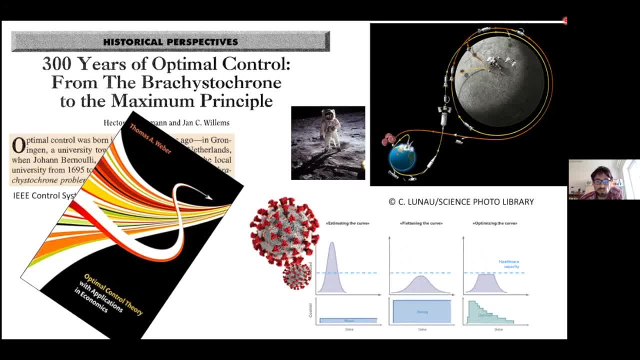 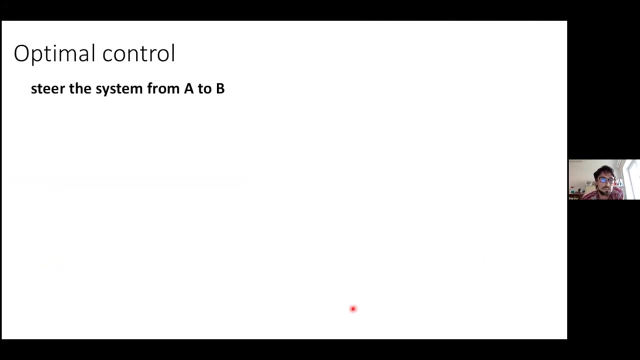 control is also the correct and well timed application of COVID did different tools to regulate the this now very famous COVID. COVID curves with, which is also, then, just problem of optimal control. So, optimal control, we may imagine it just as a tool to steer system from the point A. 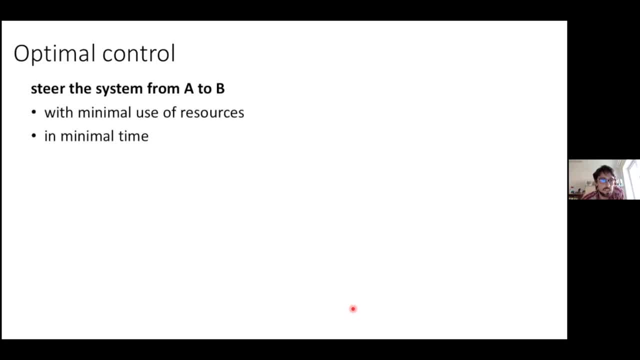 To point B and, using minimal resources, Also in the shortest possible time and following the given constraints, We can imagine that as a parking of the car in parallel park place, which means we have state A, which is the car on the street, and state B, which is the car well parked along the street. 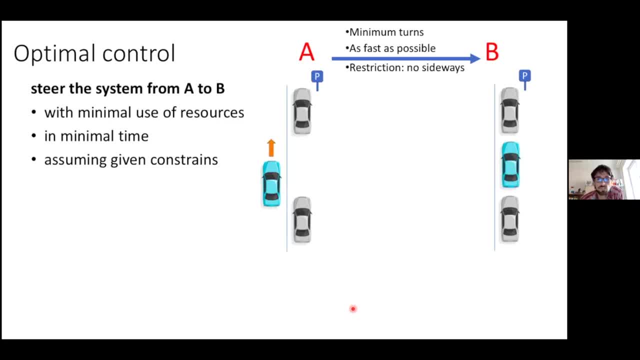 So we have. we want to do minimal turns with our steering wheel, We want to do it as fast as possible And of course, we can never drive on the side. So if you are an expert in parking, you can do it just just by as it is, but if you are a rookie, you can easily end up with such a solution, which is by far not optimal. 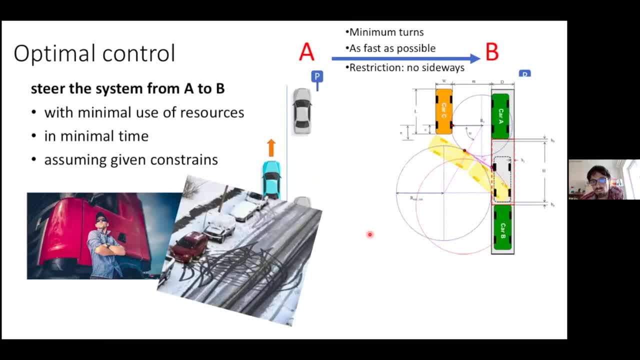 So sometimes it's better to take this problem like mathematically: describe the process and with the tool of optimal control. You then find the correct Solution under given constraints, with the minimal resources to park your car and technically you then you then don't need to steer wheel at all. 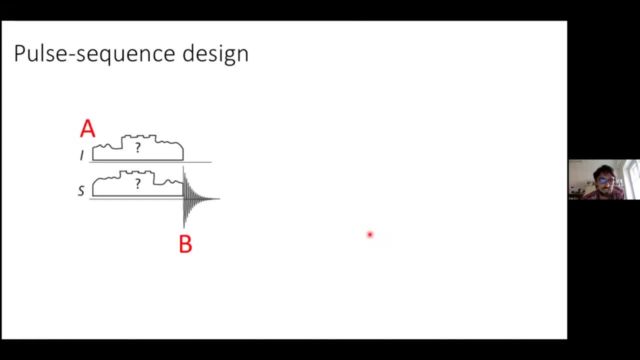 Actually, in NMR it's more or less the same: you have to state A, which may be like magnetization on one nuclei, and state B, which may be, for example, observable magnetization on another nuclei, And you want to design some pulse sequence, some set of pulses, to do this transfer. 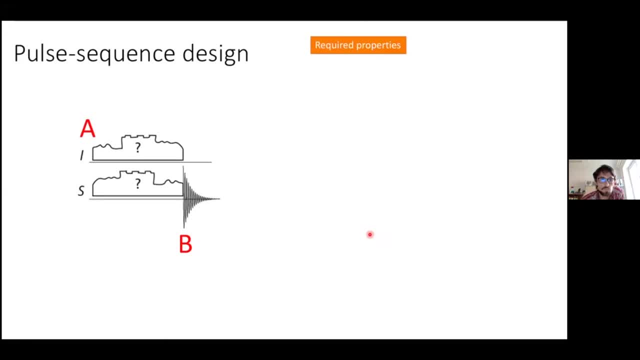 To do this to, to do to deal with this problem. So you have some required properties of this sequence and by some intuition or your experience or expertise, you design a new pulse sequence And then you try to understand or describe the evolution of the system, understand how it works and if it works well, you have new experiment. 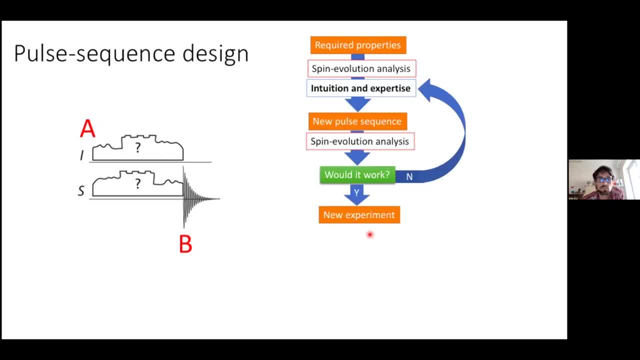 If it does not work well, you go back and again With intuition and expertise. you design a new or better pulse sequence. Finally, if you are satisfied with your experiment, you do some testing, and if even this works well, you are fine and you can publish new paper. 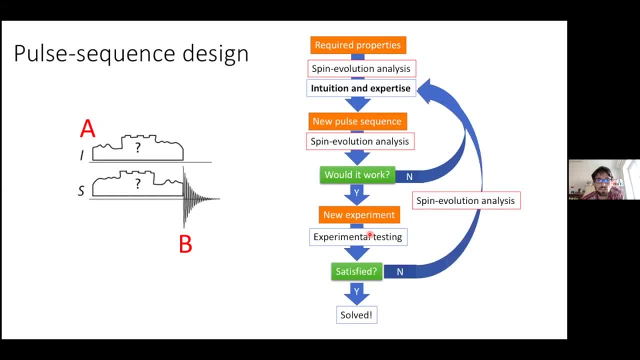 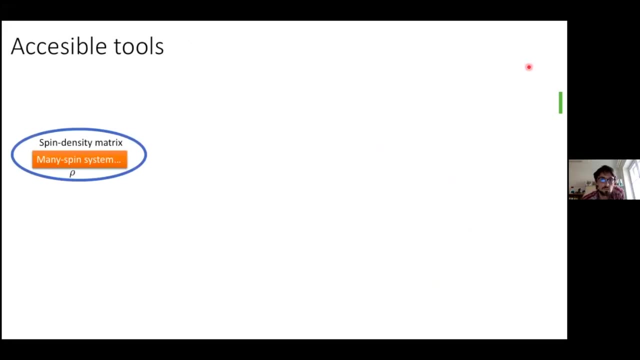 If not, you go back to intuition and expertise and try again. try it again from scratch or modify your solution. So, of course, our fathers and grandfathers developed many of useful tools for that: To: to describe the spin system with the spin density metrics, to understand or handle with different interactions using product operator formalism, which is finally sufficient toolbox for solution state NMR. 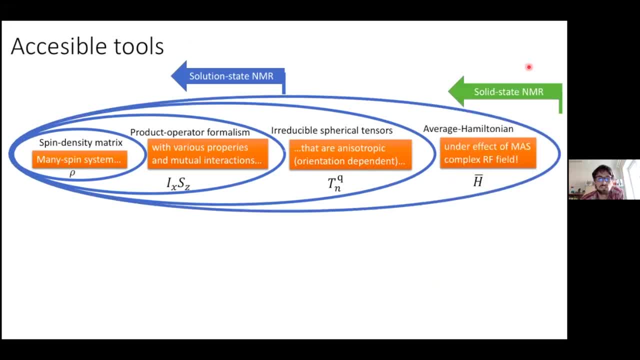 And then Transferred to every super spherical tensor space or apply average Hamiltonian theory to to work well in the solid state NMR. But unfortunately all These tools are actually, with the increasing complexity you actually increase the number Increasing complexity of the problem. you actually increase the number of approximation in your 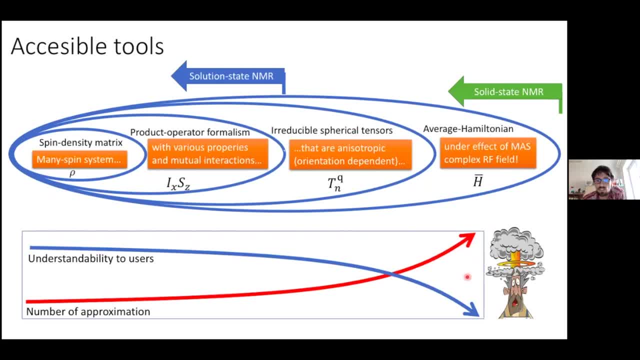 In your system, in your description, and in the same time it's starting to be really hard to understand for users. so you then ends up with some numerical simulation of your spin system using Simpson, spinach or other available software On the smaller supercomputer. 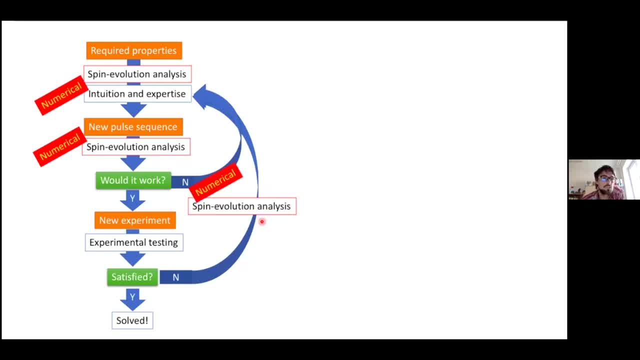 So in this traditional approach to find the new sequence, you then several times use some numerical simulation as well. so let's change the problem. let's This cup in different way, taking state age to stay, be just having evolution, evolution function, some equation of motion which can be either block or Louisville for normal. 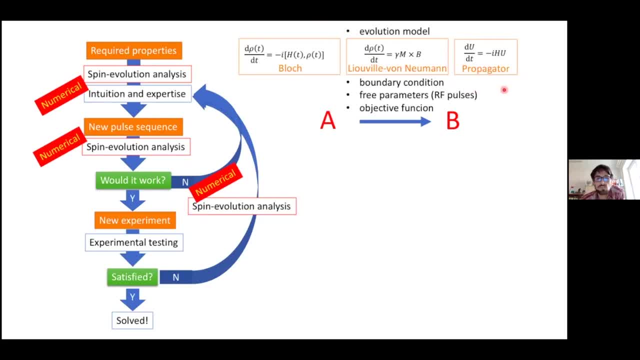 In this traditional approach to find the new sequence. you then several times use some numerical simulation as well. so let's change the problem. let's This cup in different way, taking state age to stay, be just having evolution, evolution function, some equation or it's propagator equivalent. you have some boundaries. you have three parameters which may be applied to the federal frequency policies and their their face. 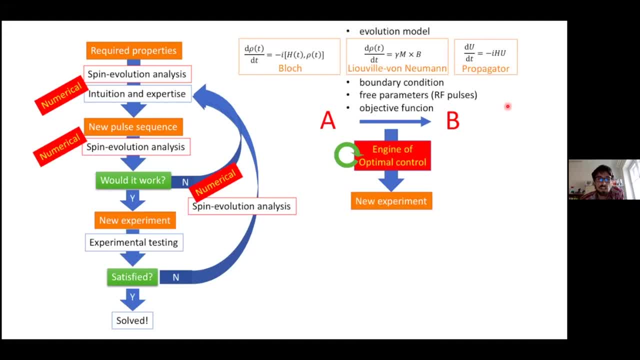 And you have some objective function, objective function, and to start this engine of optimal control which designs for you the past sequence with the correct properties under given restraints. so you have your new experiments, you tested experimentally, And you have some objective function, objective function, and you start this engine of optimal control which designs for you the past sequence with the correct properties under given restraints. 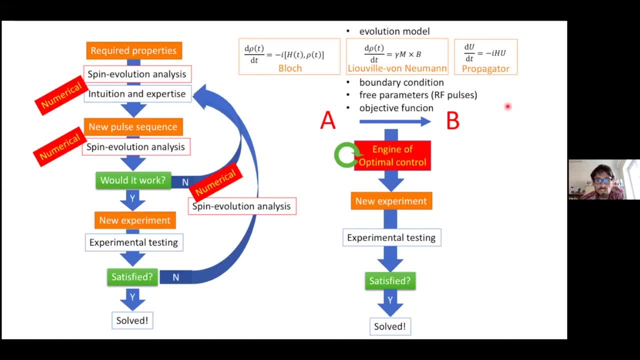 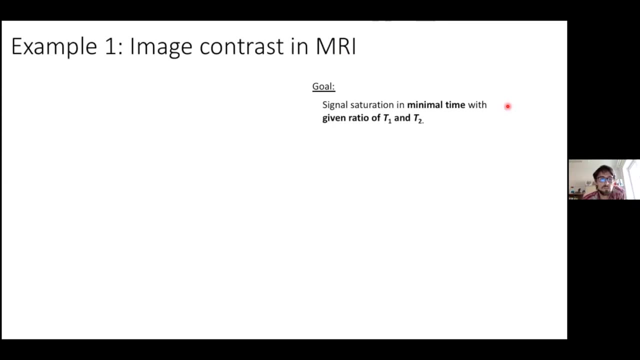 you are satisfied, you can use it. If you are not, you go back to your model, to your boundary condition, and do it again, which finally may require even less numerical simulation than the traditional approach for the pile sequence design. So first small example is this question from: 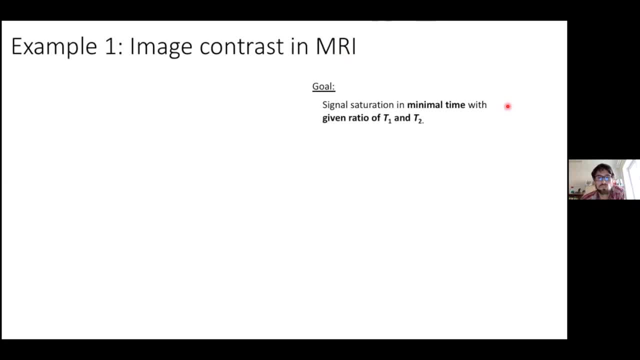 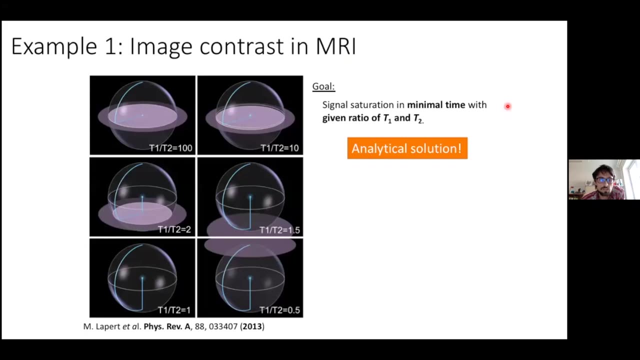 magnetic resonance imaging. The goal is to find the minimum required time, so to make a saturation of the signal in the minimal time under given ratio of T1 and T2.. This problem is in the block frame. it's actually so simple that you can find analytical solution. 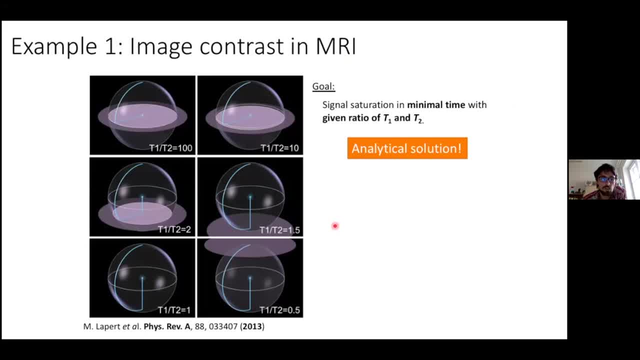 and for a different ratio. you see how long you should let to, so for how long time you should use the T1 relaxation and for how long time you should use the T2, depending on the ratio, to be as fast as possible with the saturation. 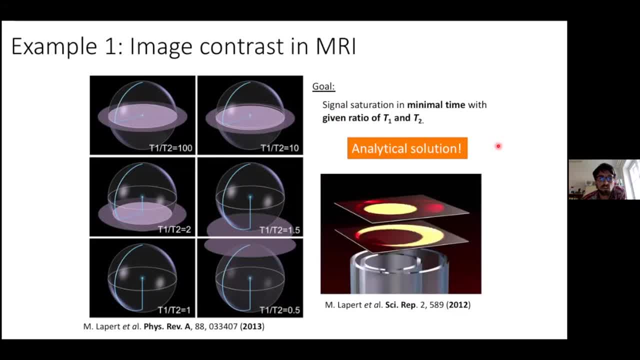 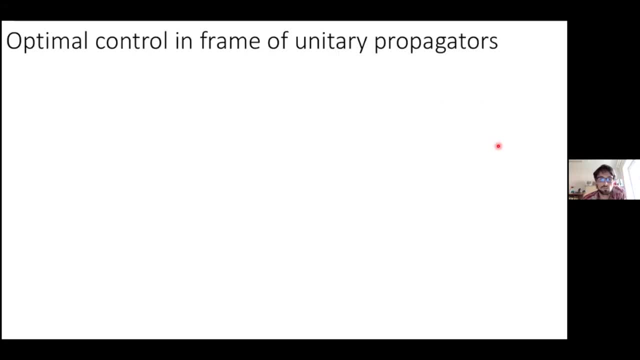 And this can nicely help to distinguish signal with different relaxation rates. in practice, Of course, block formalism is not sufficient in all cases, so I will go in details how optimal control works in this frame of unitary propagators, which is quite handy in the 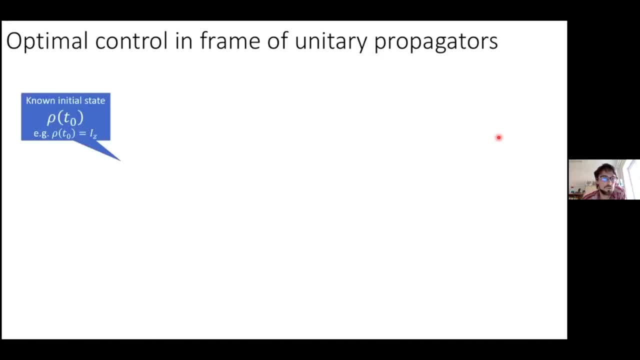 case of solid state NMR. So in the beginning we have initial state, which can be described as a row T0, and then we have now unknown pass sequence which is like some RF field modulation, and you want to end up with some desired state chi tau N. So our evolution function equation of 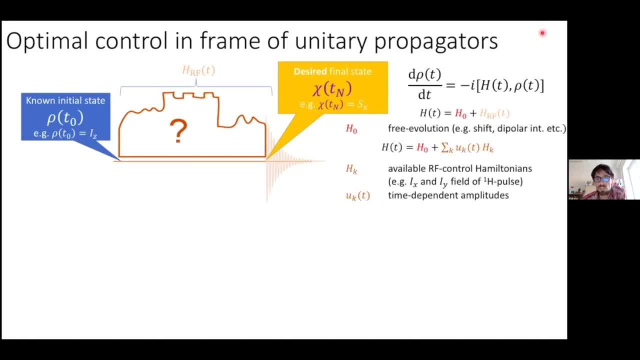 of motion is Louisville from Neumann equation and we can the Hamiltonian present. there can be split in the, in the free evolution Hamiltonian, where you have all the interactions, your chemical shift, dipole interactions, quadruple, quadruple r couplings and whatever, and then the rf control. 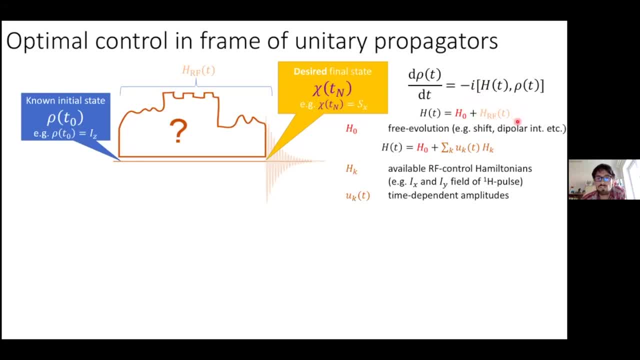 Hamiltonian or Hamiltonian of radio frequency field, which can be arbitrarily split into some time, dependent amplitudes and the and the and the Hamiltonian describing the rf field, different component of rf field, for example ix for proton or whatever. in practice it's, it's. 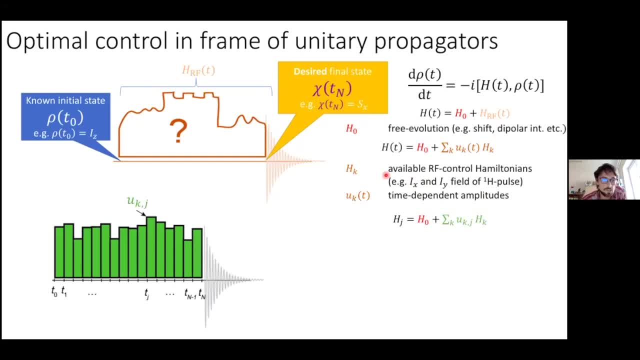 it's useful to, to take your sample, take your pulse like, take your pulse sequence as a, as a as a many small shapes, shorter pulses, which goes one after the other, and then, with this discrete description of past sequence, you can, you can describe it as a sum of discrete elements for each of that. 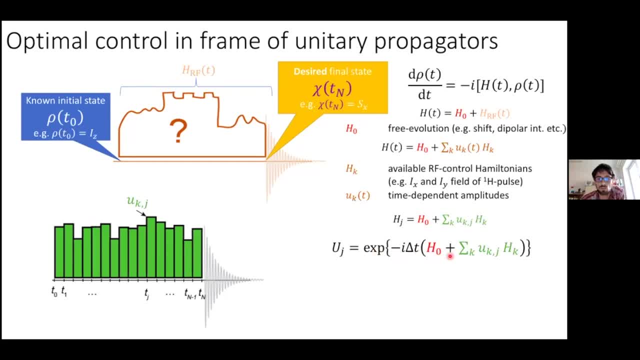 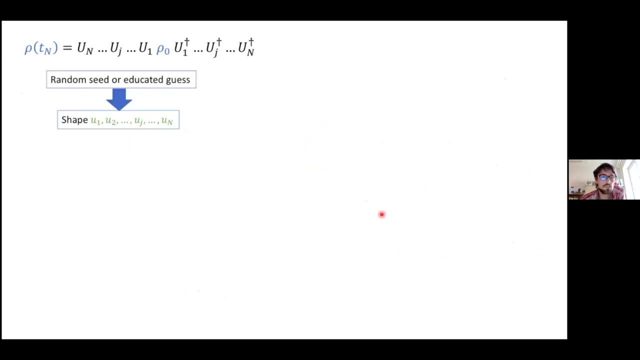 element. you can define the propagator as exponential of this, this Hamiltonian. and finally, with applying all this propagator to to your initial state, you, you can calculate your, uh, your final state, or depending on what is your actual past sequence, So the if you go farther. so here is the evolution and the algorithm of optimal. 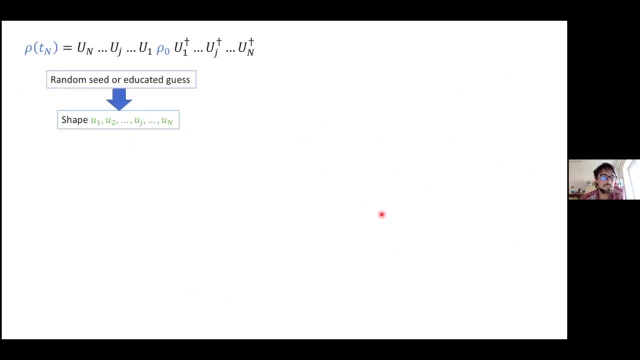 control actually starts with some random seats or educated guess which gives you some shape. so just a set of amplitudes in each time of the pulse. having that, you can simulate the evolution of your spin system and calculate the final state. if you compare the final state, this: 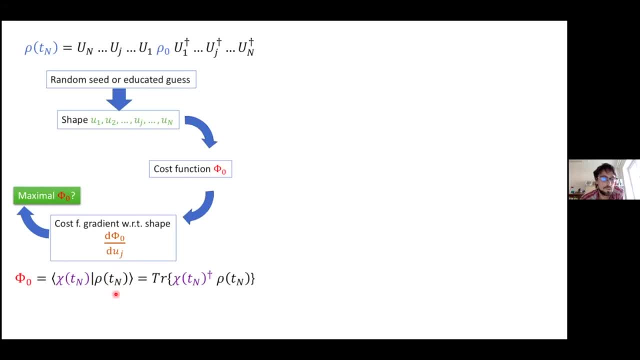 rho tau n tn. with your desired state, which is this chi tn, you may get something called cost function, or something that we would call cost function in the in the subsequent talk, and this cost function actually describes how far you are from optimal solution. so if you can get the gradient of this cost function with respect to amplitude of elements in your 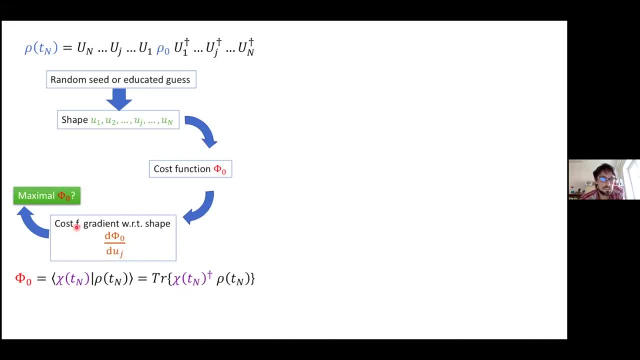 pulses. you can minimalise, you can change the, your shape to minimalise this cost function. if it is minimal, it- or sorry- maximize this, uh, this overlap function, so minimize the cost. uh, if it's uh, if this function is maximal, you are fine and you can. uh, you can use the shape. if not, you go ahead, update your shapes. 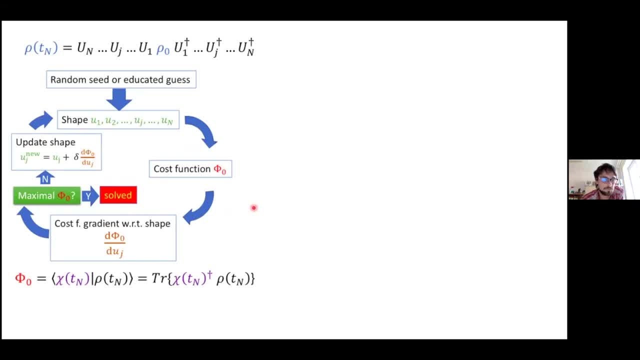 and go and go and suck circles again. so technically it's possible to use numerically calculated gradients, but then for each of the amplitude you would need to calculate to run one of these simulations and if you have like some reasonable shape with which contains, like, for example, 500. 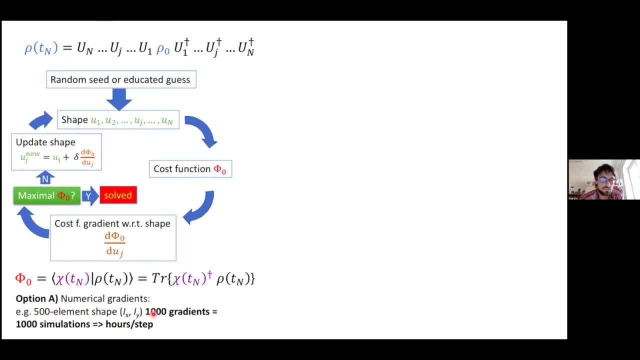 elements, then each simulation takes like approximately seconds. so it will takes an hours to to actually calculate the gradients and do one update your, of your, your shape. so it's extremely unpractical. but we can do it in in more, uh, more clever way. we can rearrange this cost, function, uh, this. 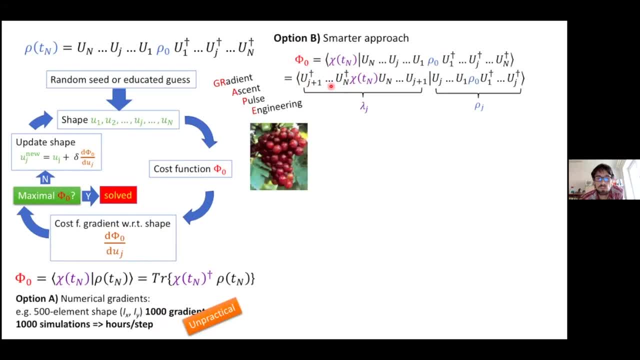 this propagators can be part of can be applied also on the on your target chi tau n function and from this forward and forward propagation of initial state and backward propagation of the of the desired state. you can calculate the gradients for all the gradients, uh for your target function. 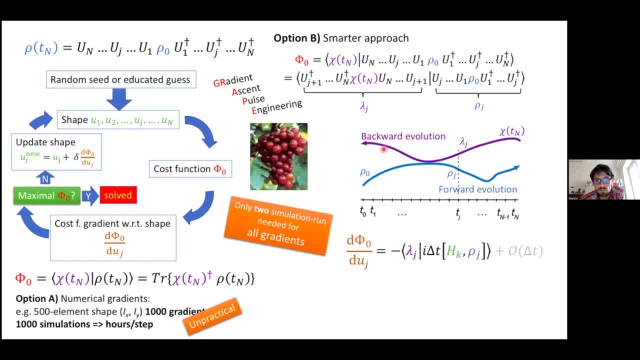 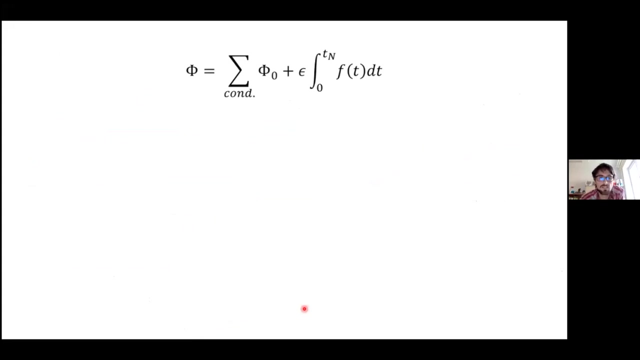 in just in just two rounds comparing these two evolutions. so it makes this algorithm extremely fast and if you, if you also apply some, some improvement for that, you can really easily get to the optima, even with the pulse which has thousands of elements. so in this one is, in this point i would like also to highlight that your cost function. 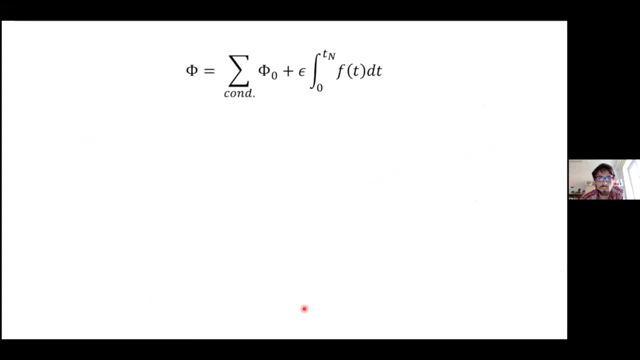 or your target function may contain, may contain more restrictions. there may be this: this terminal cost which describes actually, uh, what we have shown previously can be, can be sampled over different crystalline orientation, which makes the technique useful for design of sequences in the powder sample in solid state. you can also sample it over or sum up. 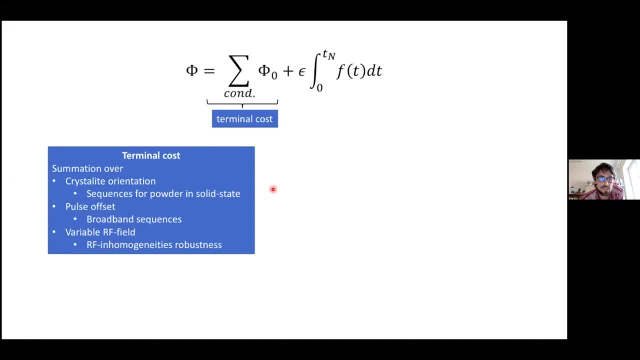 over a range of offsets, which makes the final sequence broadband, and you can also have a look on variable rf field, which then results in a sequence which is robust against the rf inhomogeneities or other effects. additionally, there is some running cost, which typically contains maximum. 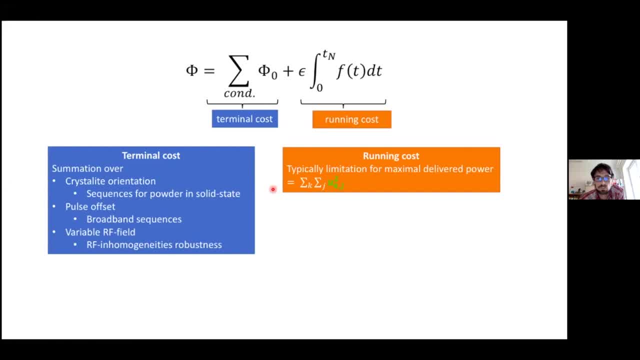 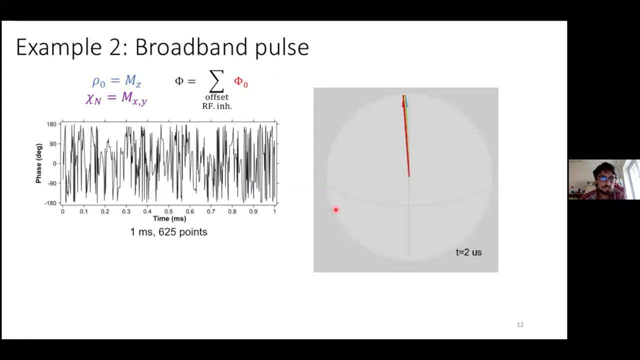 which restricts the maximum power which can be delivered by your spectrometer, by a probe to your sample, to avoid, to avoid practicality. so this is a little problem. typically it's, it's just some of the square of the amplitudes. so next example: in this work authors looked for the broadband excitation pulse, so the 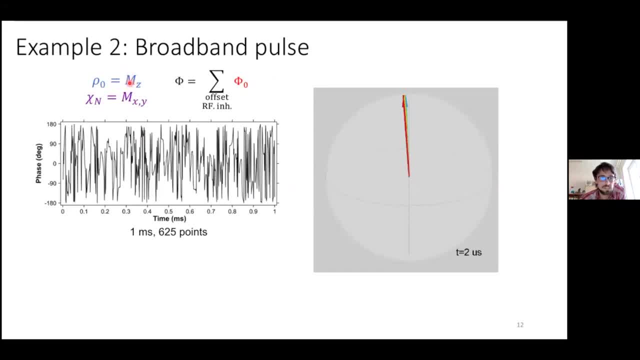 the initial function was magnetization in the z-axis and pardon, and the desired function was magnetization in the in, y, x, y plane, and so their the target function was summed over different offsets and as they want to have pulse also robust against miscalibration of the rf field, they sum up over over many rf fields. 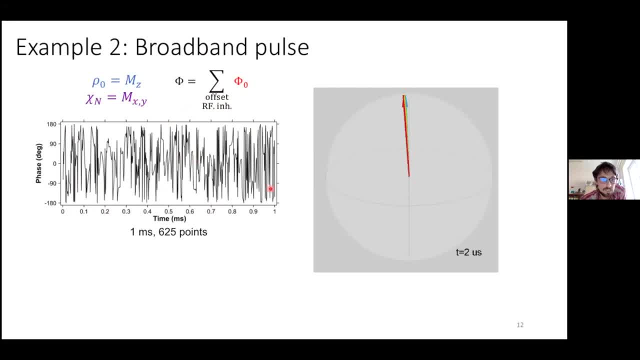 so the final shape looks is looks like kind of strangely modulated noise but it works well. i will show you in the animation soon how. but the efficiency is over 99 percent using actually any amplitude of the b1 field from 10 to 20 kilohertz and any offset of your signal. 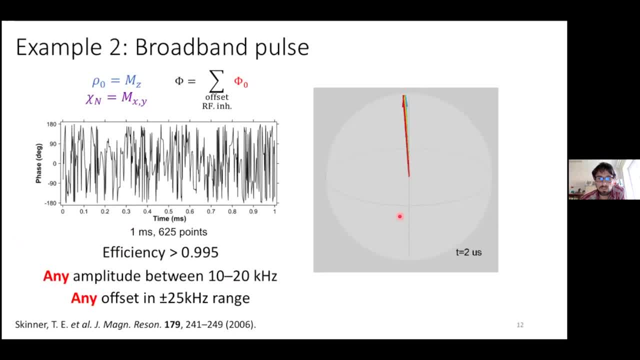 in plus minus 25 kilohertz range and i will show you on the animation if it would work. okay, so it does not work. sorry, but in this animation you could have seen that different magnetization have a completely different pathway using this shape pass, but they've all of them finally ends up in xy plane refocused. so 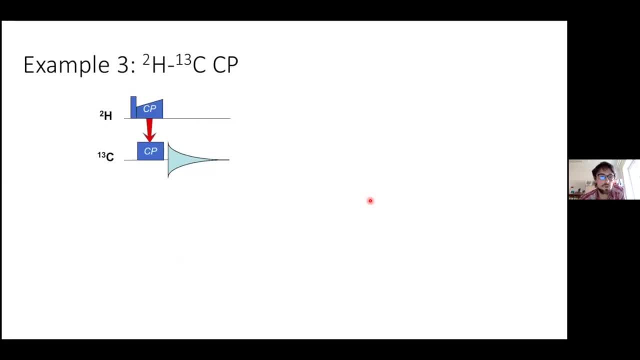 now let's move to the third example in this first block- and it would be more practical in meaning of simpson usage- and we'll focus on the deuterium carbon cross polarization experiment, which may come handy in peri-deuterated proteins, where you have much more deuterium atoms than 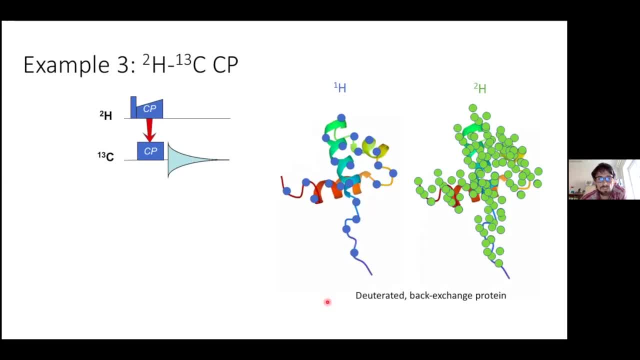 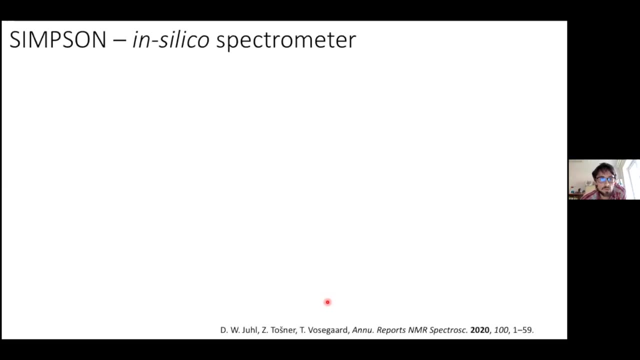 protons so they can be useful source of monetization or useful source of information about assignment or whatever you want. but generally it's difficult to perform cp with quadrupolar nuclei, so we use full in silico spectrometer, which is this simpson package in our input file we first describe our spin system as two, as just two nuclei, with some 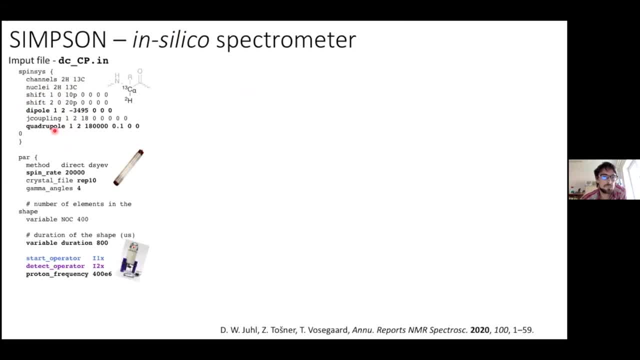 dipolar couplings between each other and some quadruple coupling on the deuterium. we also state something about the sample itself. so it's how fast we are spinning- it's 20 hertz in this case- and how many crystal orientate crystalline orientation are present in our 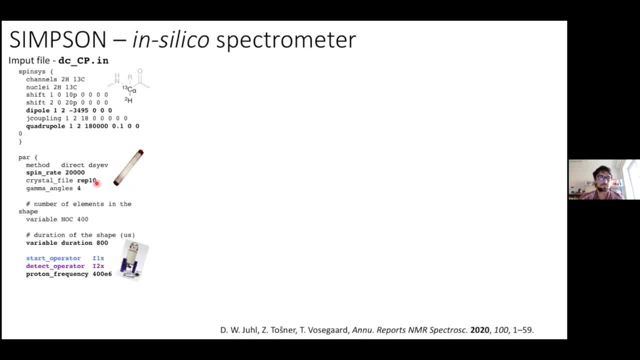 in our rotor to correctly sample the sample, the powder, actually. so then we also decided how long should be our pulse. in this case it would be 80, 800 microseconds. and then we, just then, we, yeah, we should also say what is the basic frequency of our spectrometer. 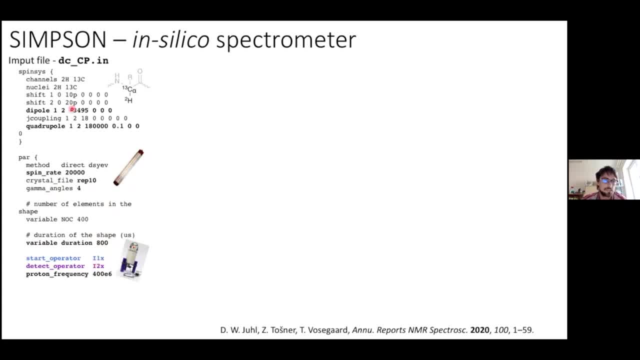 and what is the starting operator? in this case it is the magnetometer, it's coherence on the, on the div term, and desired operator is coherence on on carbon. afterwards we just state some parameters of the optimal control algorithm. so which method we want to use and how many iterations, also a little bit how big steps we use. 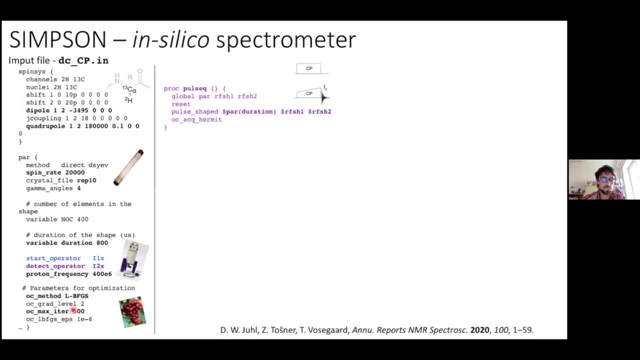 but that's all what we need to need to set up for the algorithm. and here is the pulse sequence, which in this case, is just one shaped pulse with known duration, and this and these two shapes, which are not known yet, but we are looking for them, of course, we need to state how Simpson should calculate the target function. 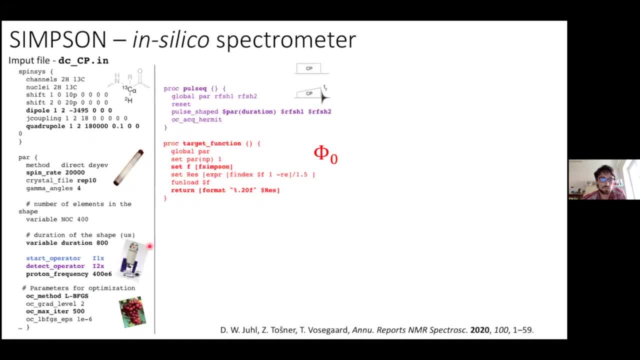 in this case it's C simple. it's just projection of the final state to the of the detected operator to our, our desired state, and similarly we did we describe how it should calculate the gradients. these two sections actually allows us to modify them to make more complex, more complex, desired. 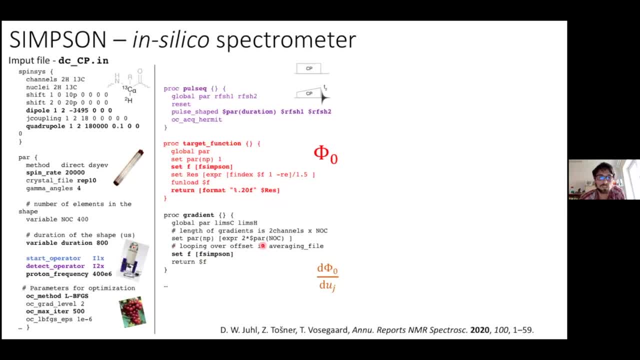 transfer, so whatever. but this is just simple example of one transfer from one nucleic to the other. so also the cost, function and gradients are quite simple. as we want to have broadband solution, we sum up over the several isotropic shift of both nuclei with this part of the script. 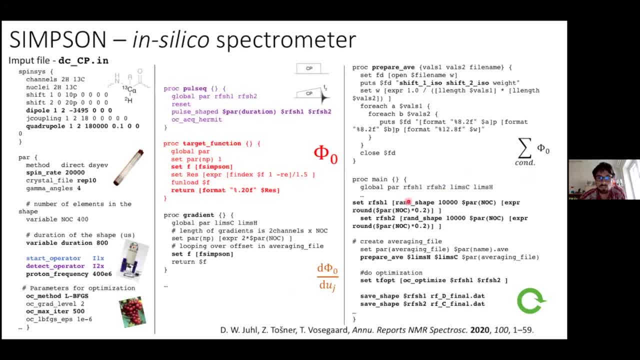 and that's all. then we can put just the section where everything's run, where we generate the random seed on the beginning and may prepare some list of of chemical shift for this sum and finally- sorry, i didn't see this over there. yeah, and finally we just run the optimization and save the shapes, that's all. 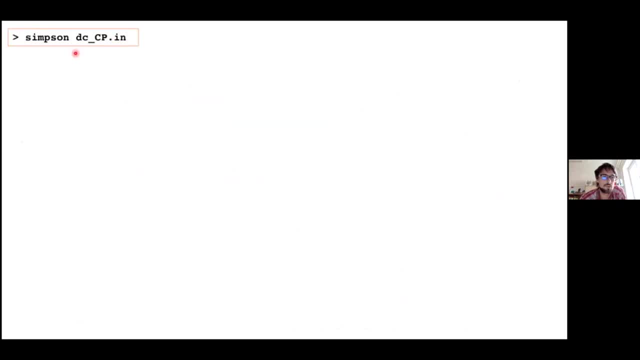 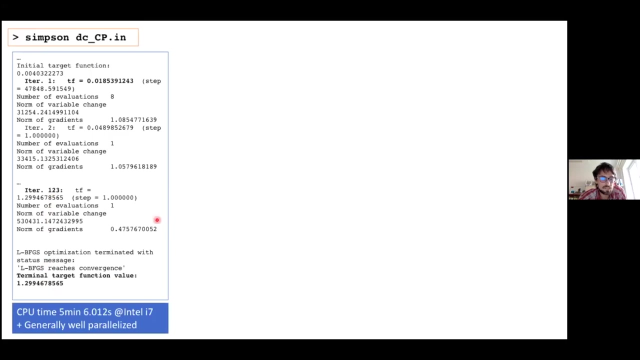 in command line. we just wrote simpson and our input file and we get some information that we can use in the optimization procedure. it takes some a bit over 100 iterations to get to the maxima and the. the target function over then is like 1.3 and we get these results in. 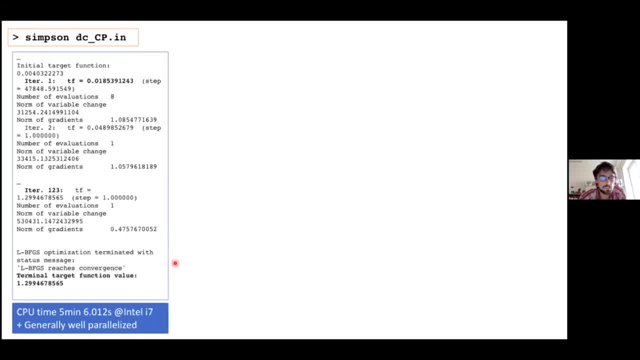 like five minutes approximately. this simple is. this example is relatively simple, so it's it can be PC. but all this problem is generally well parallelized, so it can be also for more complex problems. it can be easily used on the clusters or supercomputers. so this is our resulting shape. 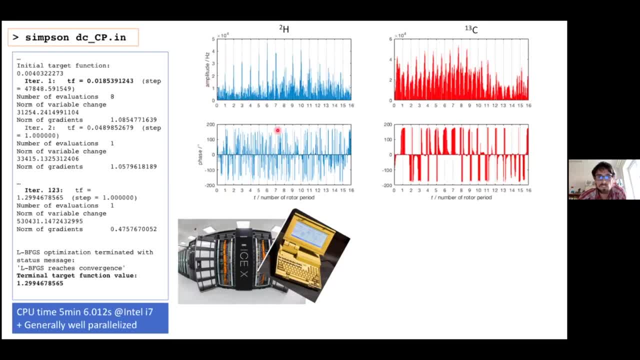 you may see that, compared to previous example, this shape actually looks quite, quite systematic, not just like a noise. and what is actually interesting is that the solution of this problem using optimal control actually inspired those authors for for the respiration cp experiment, which is described here and which contains quite similar pattern of the of the two broadband. 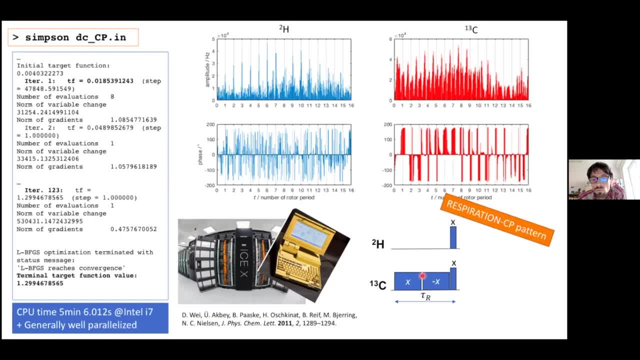 opposite pulses, two, so sorry two, two long, two long passes with opposite phase. on the carbon channel- you can somehow see them over there, and you see opposite phase here, followed by by short pulse, which is here, and in the deuterium channel you may see just the short pulse, one in each rotor period. 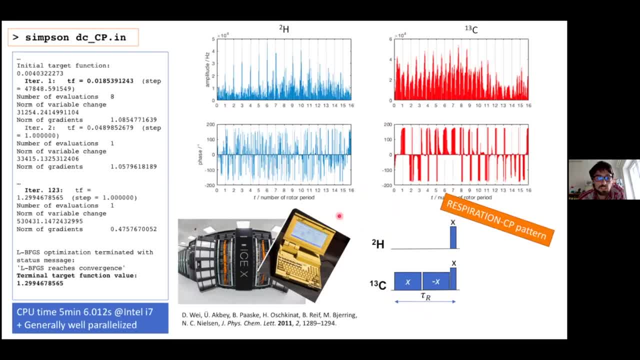 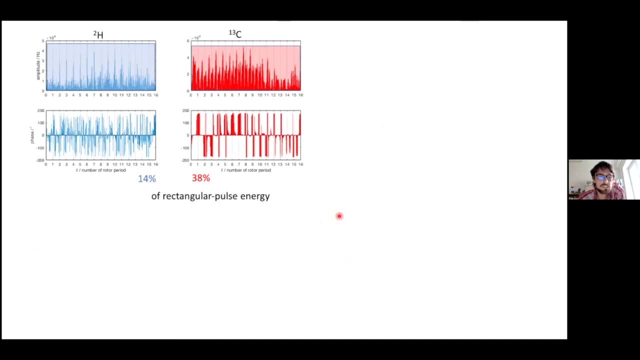 so this pulse sequence is nicely synchronized with rotation which is quite frequent feature in the optimal control based optimized pulses. so what is nice about bus sequence we just get is that compared to rectangular pulse it has really much smaller, much smaller energy, much smaller power delivered to by the probe, to the 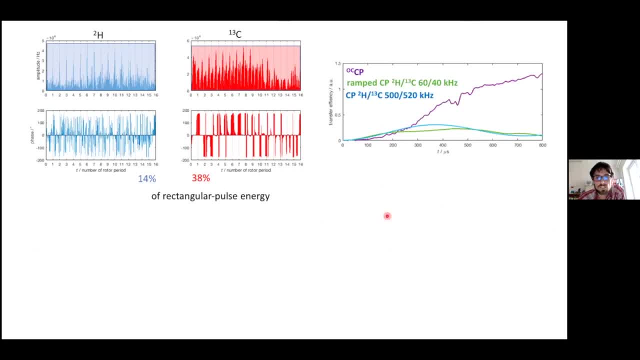 sample and also the efficiency is substantially higher. and in the violet color you can see our optimal control pulse in simulation and this blue and green color is the cp with just crazy powers for, just for comparison and ramp cp, which something closer to the optimal control solution but still the efficiency of the optimal control cp in this case. 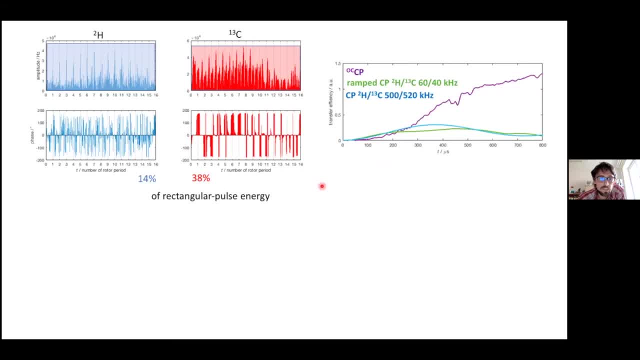 is much better, great. so having these pulses actually and we are ready to use them and they are technically for use in any 400 spectrometers at 20 cohertz s also a bit beyond that, and this is something which i will touch in the in the second part of my talk. so this was for the first part at the end. 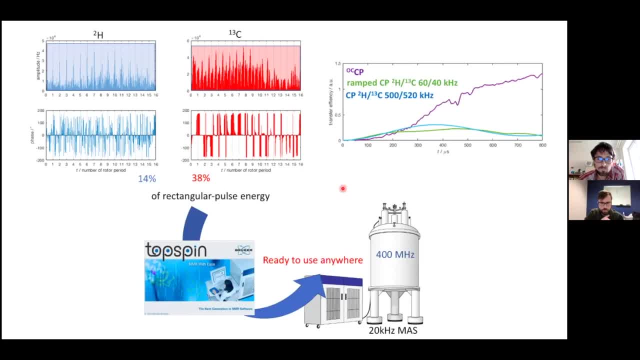 all right, thank you. very interesting first half. so if anyone has any questions, feel free to submit them through the q a function. um, we have one already, uh saying, if i understand correctly from a anonymous attendee, so it is. is it machine learning, basic gradient, descent, uh application and pulse. 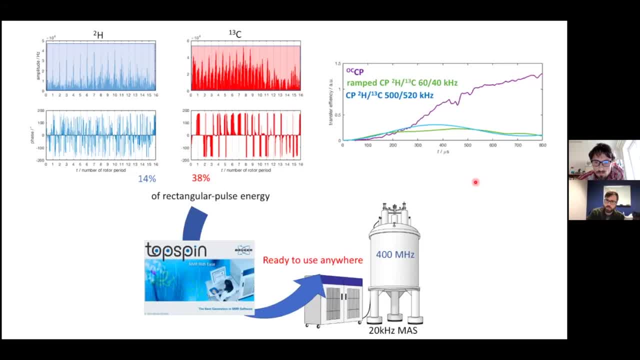 optimization. have you used any deep learning model? uh, no, uh, we haven't. so so this, this, uh, this algorithm is just just the gradient descent. uh, technically it could be possible, but, uh, we don't need it yet like any deep learning or this, this modern tools, because we know. 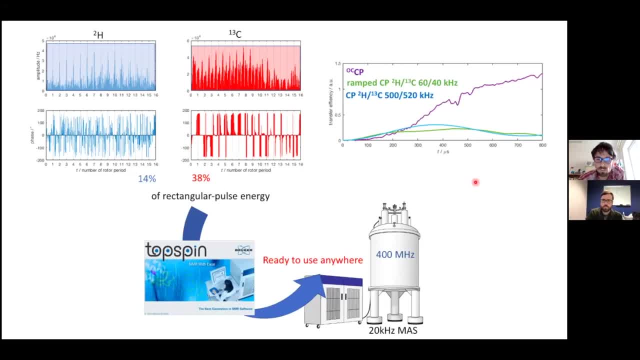 gradients. we know all the math, we know how the system behaves, so we can quite easily get to the, gets to the optimal with, with, within standard tools. and then, uh, yeah, uh, added to that question: that is not uh, this is a straight optimization theory. yeah, and then, uh, we have another question from uh. 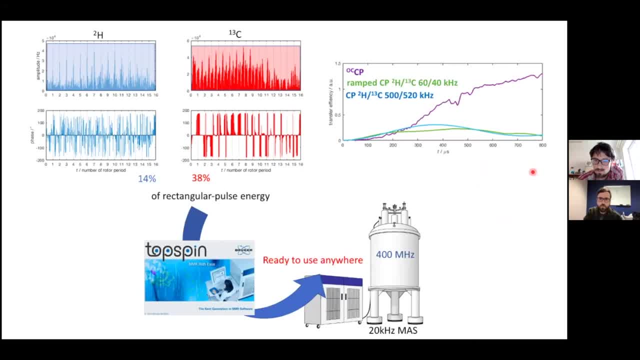 dominique masio asking: is there a unique way for defining the cost function? depends on the problem you are solving, depends for what. what you ask actually like if you, if you want, just transfer from one spin to the other in this unique way, but if you need to. 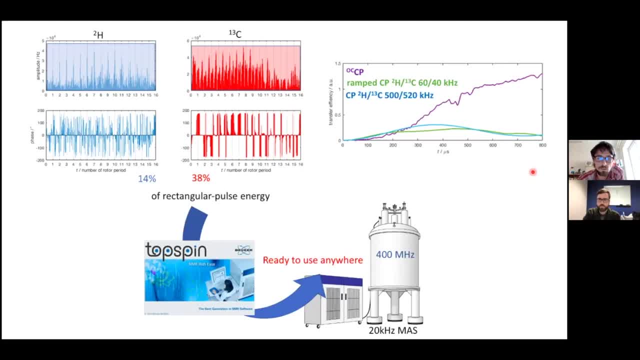 compensate your if you need to make your solution robust against some inhomogeneities or other effects. there may be several ways how to describe your cost function, So it depends for what you ask. With more complexity, there are more options to define the cost function. 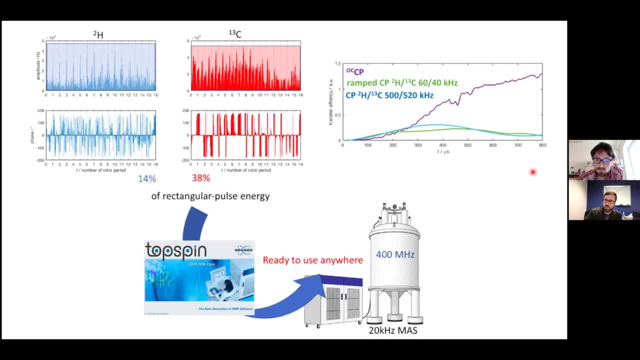 Then we have another question here from Rasek asking: is there a way to include the effect of T1 or T2 relaxation in the exercise? Yes, in principle. yes, The same algorithm can be formulated in Leuvelian space, and then you can do it also including. 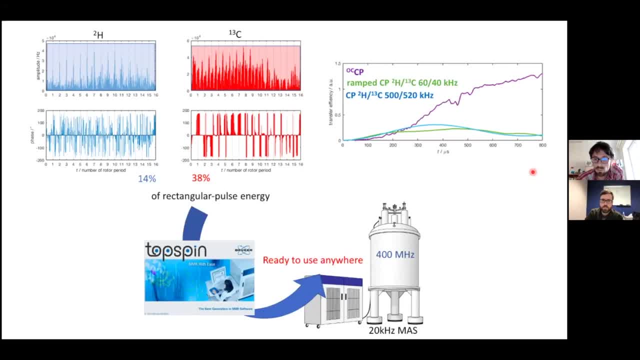 relaxations. Just, you will struggle with the problems that your propagators are not unitary anymore And you will probably need to make the algorithm a bit different for that. But technically I think it is possible. And Dominique Bastiau with another question asking: 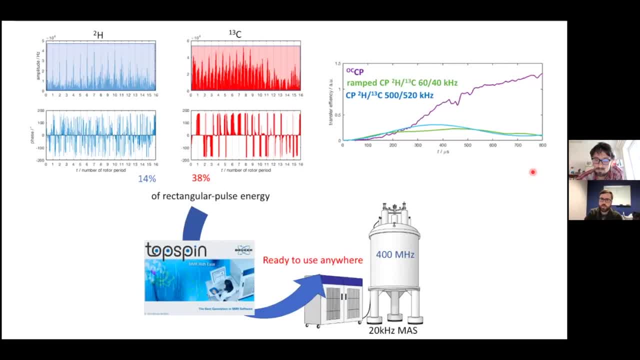 so how can the efficiency be greater than one? What is the definition of your efficiency here? So it was not efficiency, It was just all overlap of this of the initial state and final state matrix mostly, And that can be normalized in different way. But there is a different normalization here, So it depends how you normalize your problem. 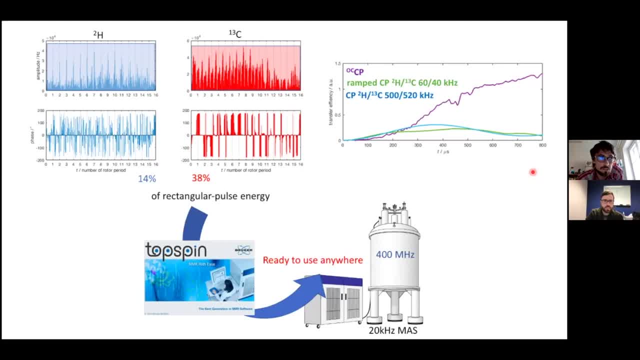 I think the normalization here was just the pure carbon magnetization. That is the reason. So we gain some, All right. And then we have another anonymous question here. This is from a student who is interested in: is it possible to apply this method to? 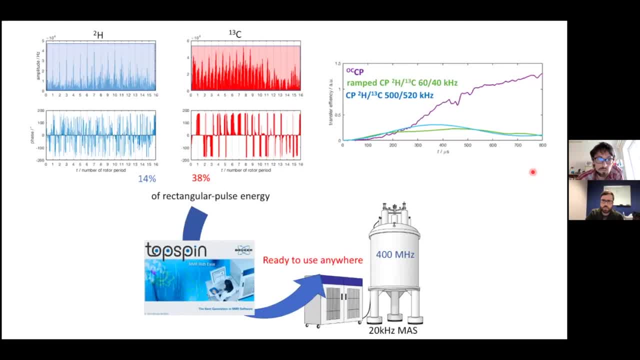 recoupling sequence design. Yes, Yes, I will cover some of the examples of that later. And in principle this is also recoupling This respiration thing, is recoupling of the diapolar coupling between deuterium and 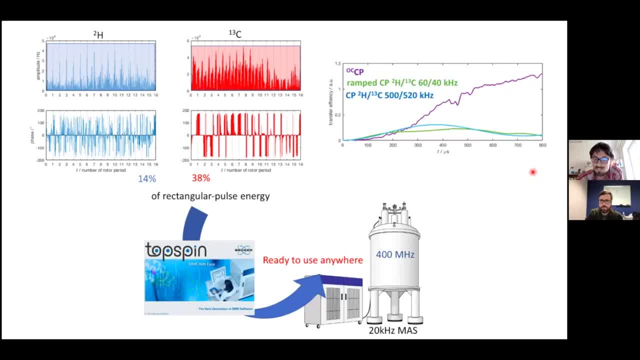 carbon. So yes, And it's frequently done. All right, We have a question here from Jörn Schmidt. I'm so sorry if I butchered that, But will you find ordinary pulse sequences by using a crude grid, or would some solutions be inaccessible by the algorithm? 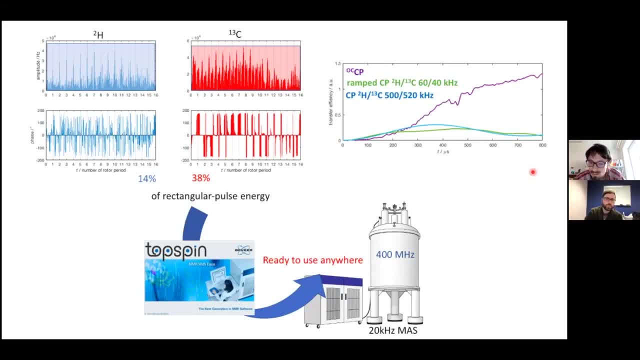 Can you read it again please? So will you find ordinary pulse sequences by using a crude grid, or would some solutions be generally inaccessible by the- by the algorithm? I think this is pointing towards how respiration kind of popped out of it. I would say that it's opposite. actually, With optimal control, we can find a solution which. 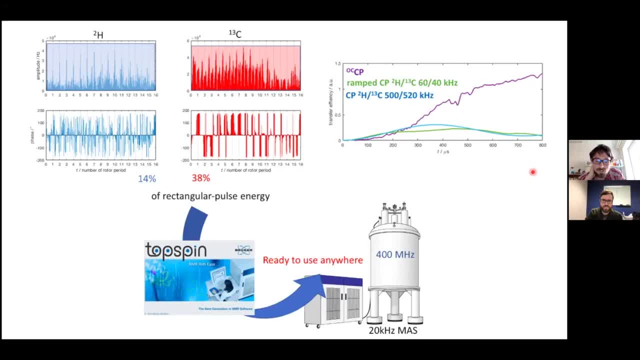 were unknown before, and we can also think about transfers, which for that there were no pass sequences before. So sometimes it happens that we converge to some known pass sequence or to some features which are known, but I don't think that something is prohibited for the optimal control If we allow the system to develop in some state. 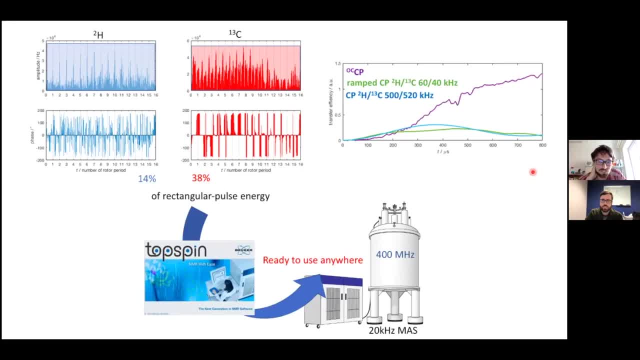 if we allow the pulses in the correct channel, with the certain amplitudes and and phases, it can convert to these solutions. If it is the best, it will probably Right. then I think this will be our last question for this break and then, if anyone, 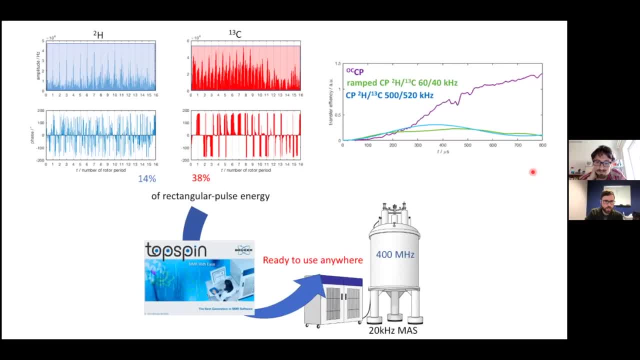 has any other questions, feel free to continue to add them to the Q&A and we will address them at the end as well. And so from Hector Cortes asking: in your examples you vary the RF while keeping the pulse length constant, but could you keep the constant RF field? 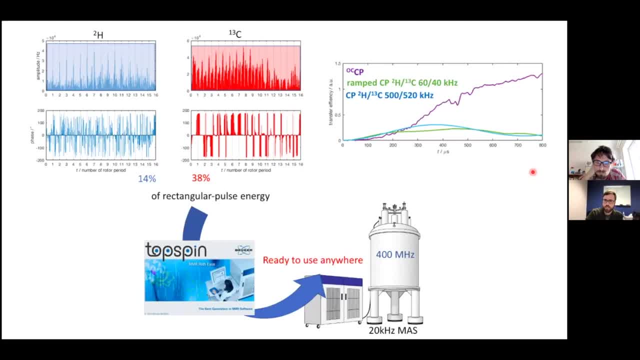 and vary pulse length, and does that provide any benefits? I think in my examples we varied both the amplitude and the phase as well. Maybe I missed something, or Could be. I think that, yeah, that was just Yeah. so if I haven't highlighted that typically both the phase and amplitude are three parameters, 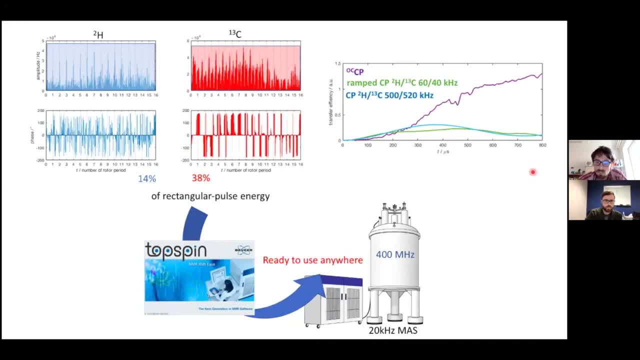 which are varied. So yeah, Maybe in the algorithm I just put the U as an amplitude, but there were always, there would always be Ux and Uy, which means like amplitude in X channel and Y channel, which finally means different amplitude and phase. It's just a matter of formalism. 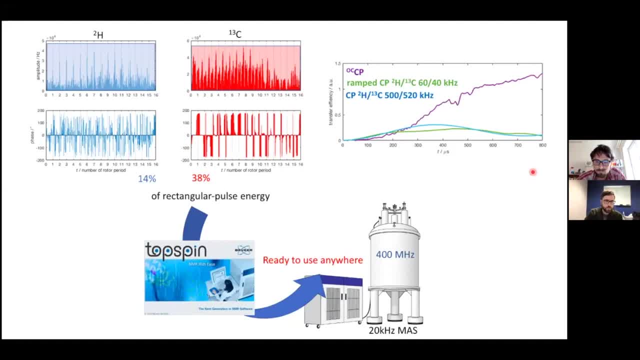 There's also a clarifying message from the previous anonymous MD saying sorry by recoupling. what they meant is like s-respdoor, but not symmetry-based sequences, where the goal is not maximizing sub-signal but measure distance, for example. 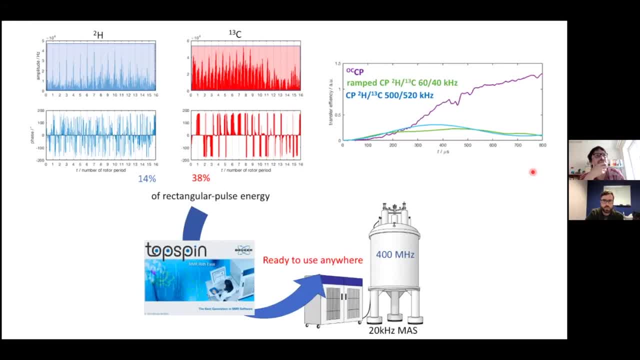 Yes, yes, technically, yes, I would just need to think how- how to make this pulse sequence reproducible for different distances, But I'm convinced that we can to formulate the correct problem and find a solution for that. Thank you everyone for your questions and I thank you as well. 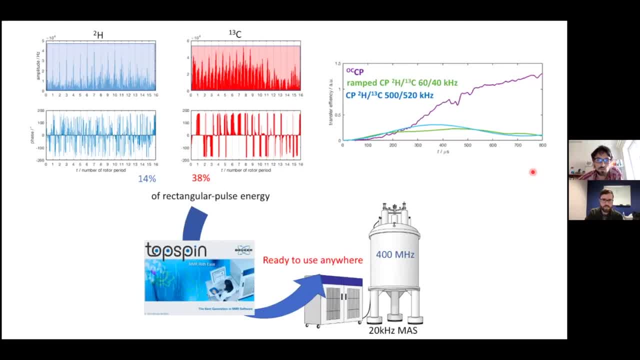 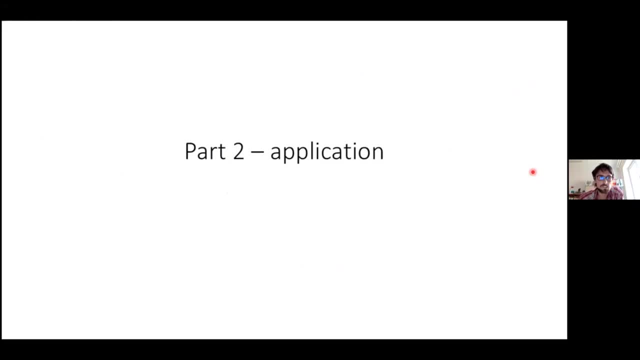 And please continue, OK, OK. so let's go ahead. Let's go to the second part with the applications and with some restrictions which our hardware makes due to our genius solutions. So first are the transient effects. Actually, the question is if the spectrometer transmits. 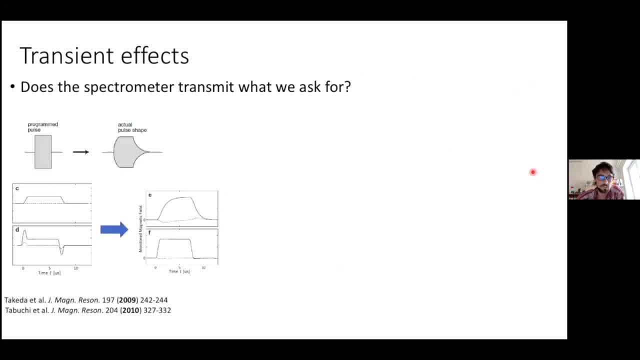 if the probe transmits exactly what we ask for. It's known that, for example, heart pulses are not transmitted in the correct shape and the actual shape of the pulse is something like that. So there were attempts, successful attempts, to make corrections, changing the shape of the pulse. so 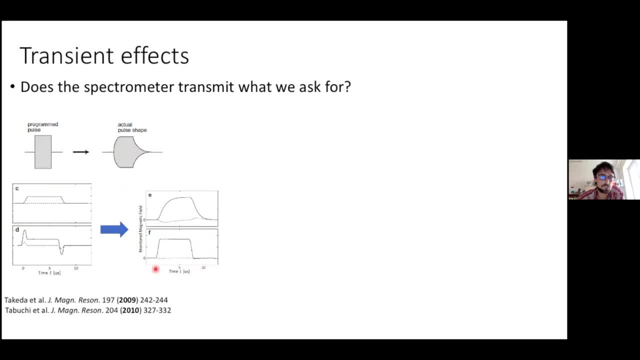 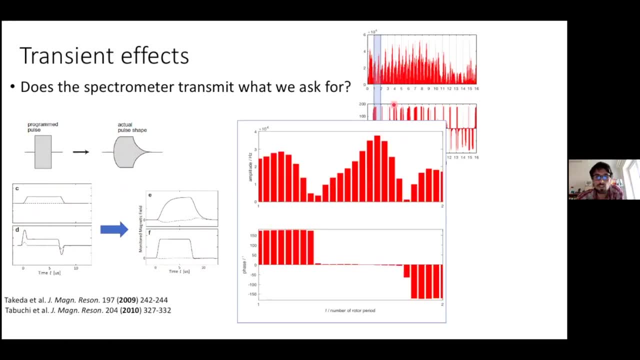 that we get as rectangular response as possible. But what about our optimal control solution? If we zoom inside, you may see that there are quite significant changes in the amplitude and also in the phase. The question is if the spectrometer reproduces it correctly. 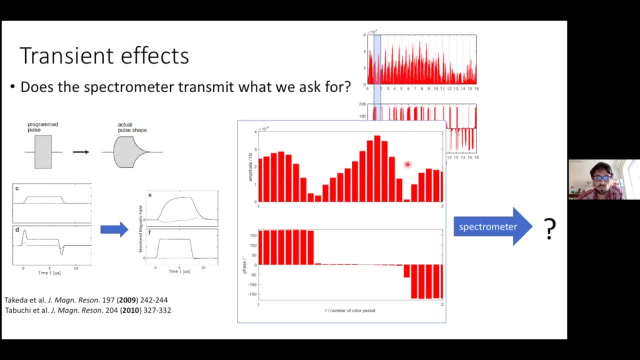 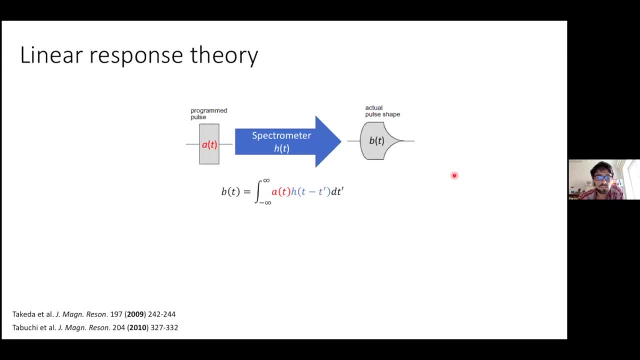 If the spectrometer correctly transmits everything what we ask. So we can use linear response theory to understand and to describe our spectrometer, using this response function h which, after a convolution with our signal, give us the actual response of the shape. So this function h is also called impulse response function and it's basically 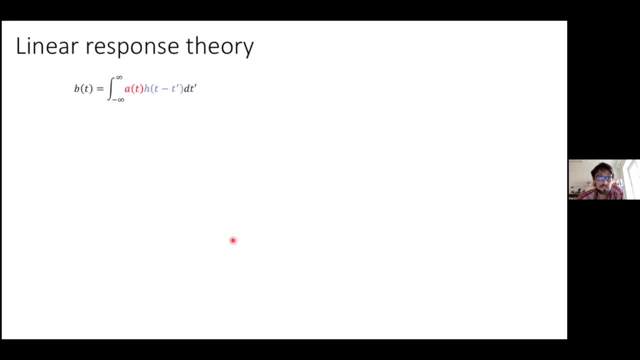 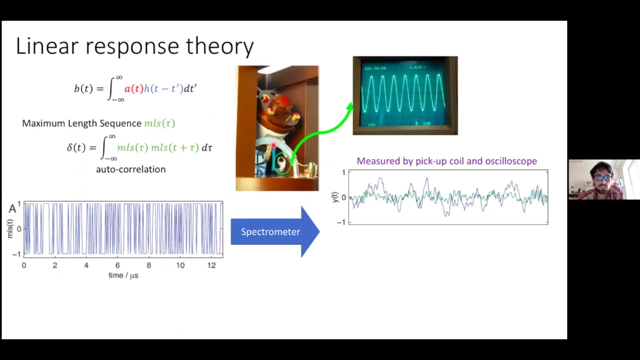 the characteristic of our hardware. It can be experimentally determined using this maximum length sequence, which is just the kind of shaped pulse with the special properties that its autocorrelation is delta function, And if we transmit this function to the coil of spectrometer and using some pickup coil, 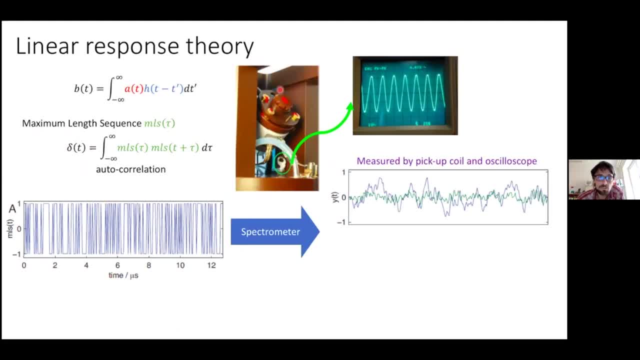 which is just the coil nearby our stator, nearby our coil in the probe, and measure the actual current in this coil, we get some function, We get some response of the spectrometer to our shape, of the maximum length sequence And if we do cross correlation, 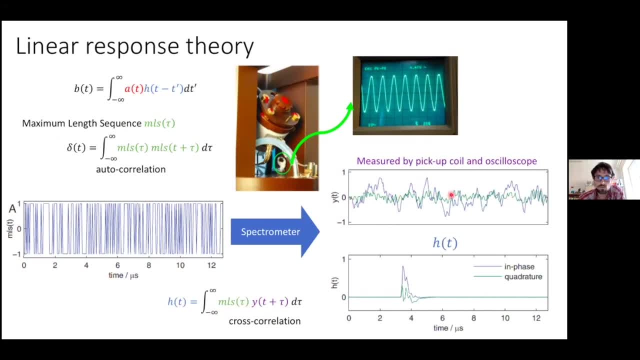 between this function, which we get from the, which we measured using oscilloscope, and the original maximum length sequence, we get this response function, And this response function can be later on used to understand what is what the spectrometer doing with our shape. 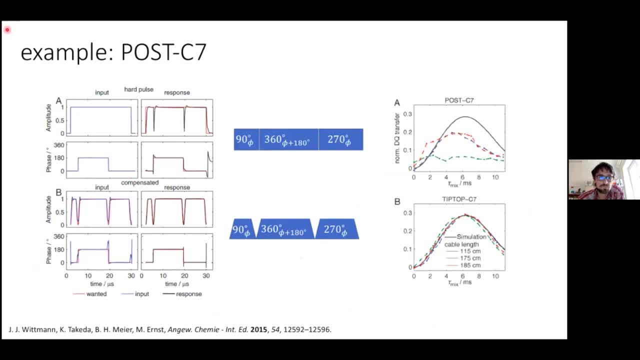 It was done also in the field of analytical pulse sequences, for example here post C7.. So we can see that in the field of analytical pulse sequence, where they found, using a response theory, that fast and rapid changes in the phase actually induce some spikes or some problems with the, also with the amplitude of the pulses. 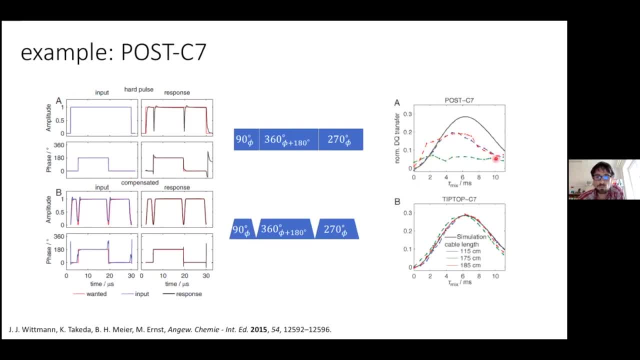 And then the results are not reproducible at all And depending on the length of the cable in a spectrometer you actually get different shape of your recoupling, different recoupling curve, let's say. But if once they compensate it, 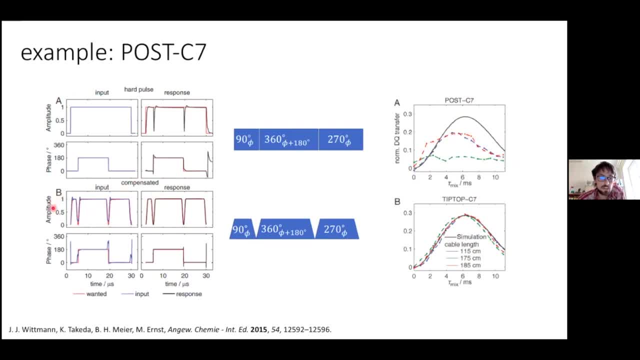 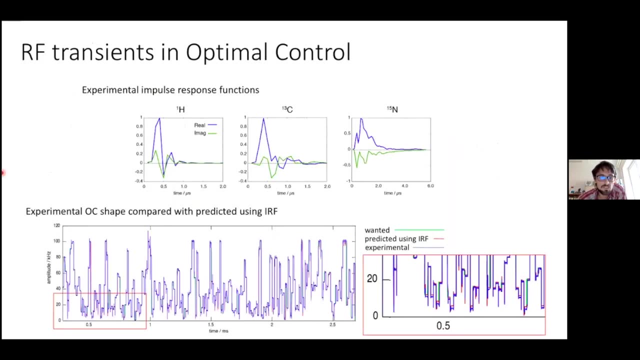 for this, for this hardware characteristic mostly, the response is now nice, Everything goes smooth and and the pulse sequence reproducibly independent. on this hardware parameter. We can have a look on the optimal control sequences in the same way. So here is for one concrete spectrometer. 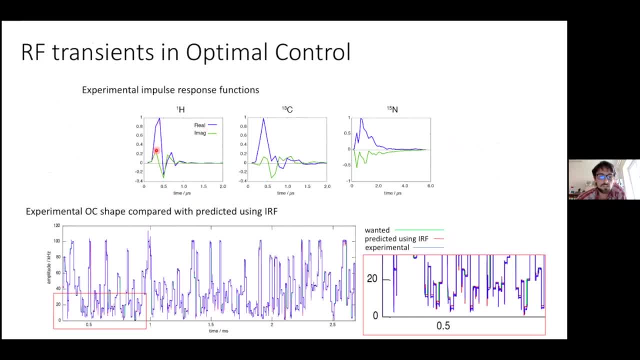 There is a real and imaginary part of this response function for three different channels And if we have a look on one of the optimal control shape and if we zoom to it, we can see that our actually experimental response is really close to the, really close to the. 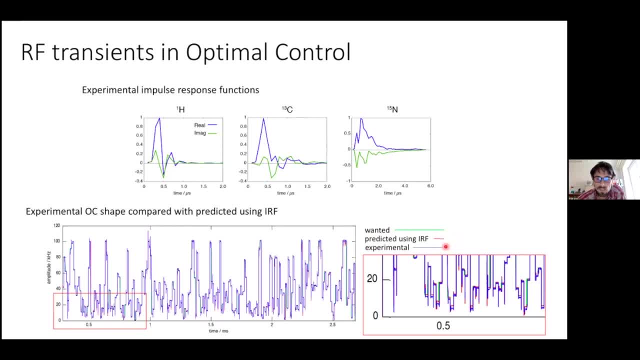 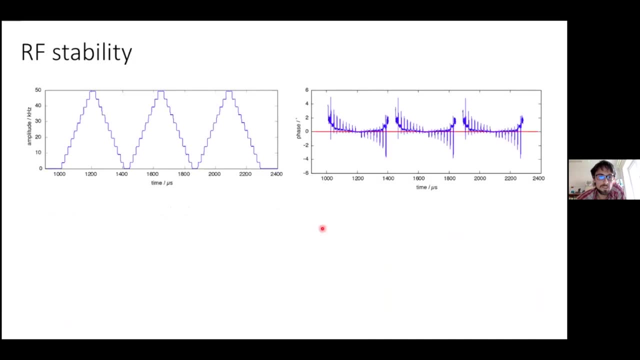 to the shape which we want And also, well, I agree with the shape predicted using this, this impulse response function, So this is not a big problem. And another experiments which somehow indicate how much is our system stable and how well it reproduces the shape pulse. 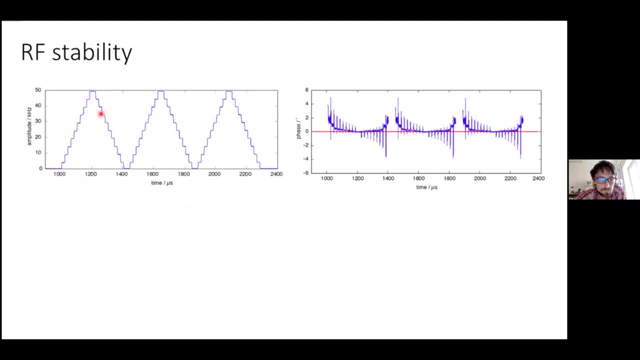 is this experiment where we transmit different amplitude pulse with variable amplitude in time, and looked, looked on that We see that there is, there is a face and so this is the experimental response of the spectrometer And we see that in any time where we change the amplitude there were some small spikes. 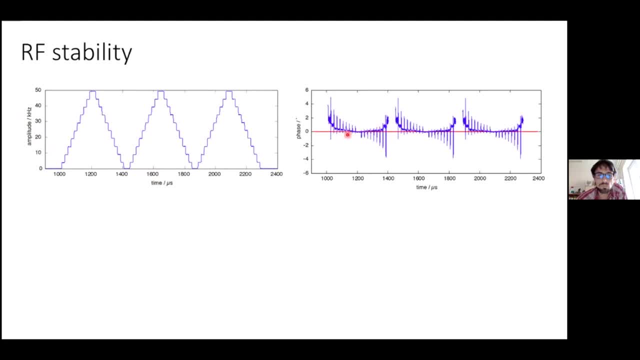 of the face, some inaccuracies, But it was mostly small. You see the wire scale here It's just just the, I would say, degree or few degrees, And also the stability in the long term. if we here have a look on the same step in different times is quite good in the most. 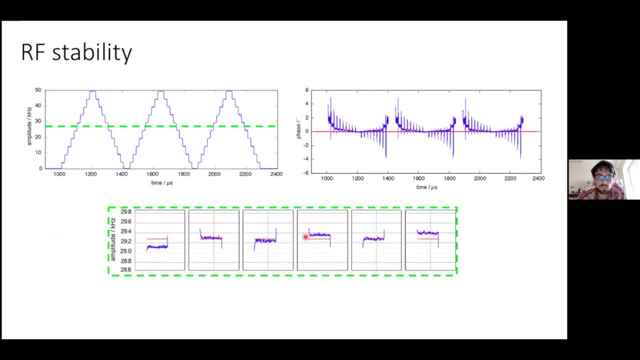 time. the red line is actually the theoretical value of the, of the, of the signal amplitude, And the blue is what we, what was measured, And you see that sometimes it's slightly smaller, Sometimes it fits well, sometimes it's gently higher, But usually we are in the in, we are close to the, to the theoretical value. 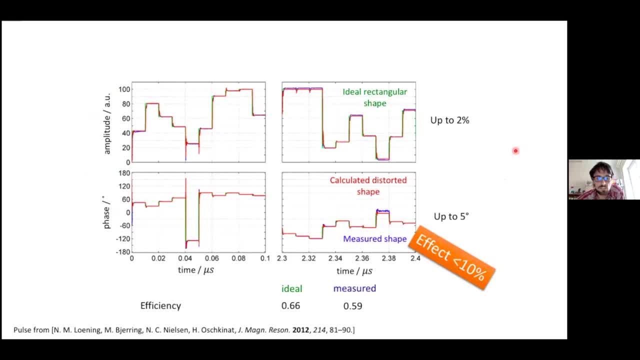 So the conclusion is that this transient effects and instabilities of the of the hardware actually makes, in the maximum case, just a few percent of the amplitude distortion and just up to five degree in the face distortion, which is exactly acceptable and in the most cases for optimal control. 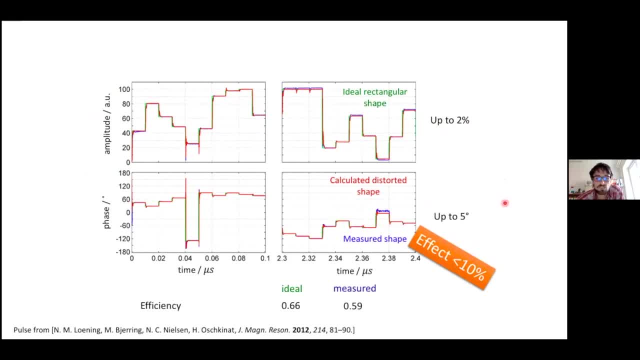 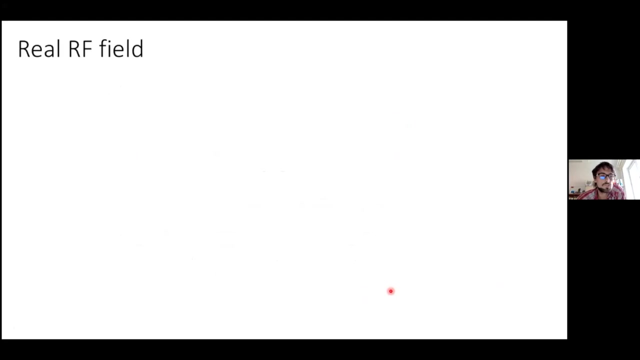 policies. the effect is, the effect in the effect on the efficiency is less than 10 percent if we compare the measured value with the ideal one. So basically, the transient effects for optimal control are not such a big problem. What is problem? usually shown recently that the RF field. 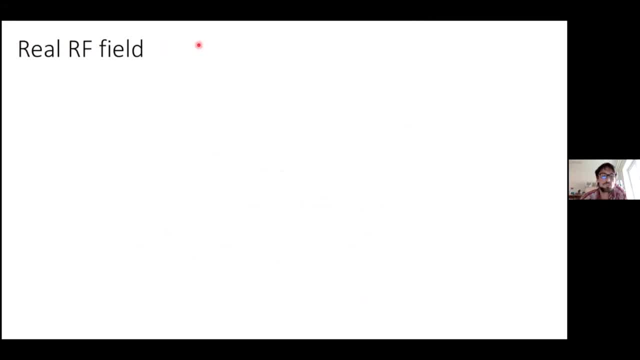 RF field inhomogeneity is the big problem for optimal control. So let's have a look a little bit in details. What is the RF field inhomogeneity? So if you have a look on the sample, you have the rotor and the solenoid curve. 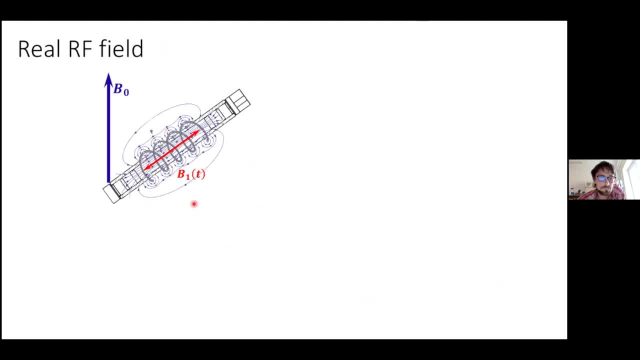 So sorry. You have the solenoid coil around that And basically going along the axis of the rotor you have some part where the field is quite homogeneous, But then on the edge of the coil you wrap, the field is rapidly decreasing. 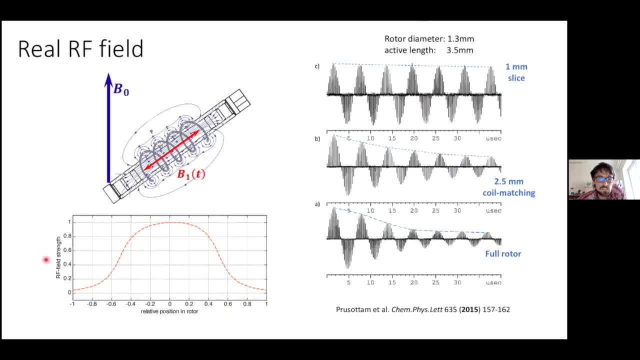 And the strength of the field. this can be seen if you do the, if you do mostly mutation experiment here. on the first, on the first graph, you see just sample containing tiny slice of the measured materials in the middle of the rotor And the mutation curve is fairly stable and does not decrease too much. 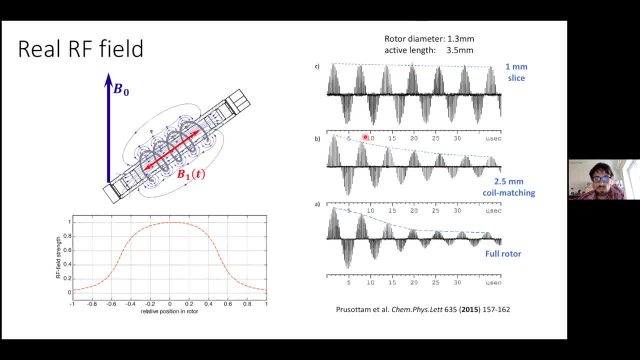 But if you increase the amount of sample- for example- here it matched the size of the coil- there is some, there is some decrease in efficiency And if the rotor is full there is a huge amount of signal in the beginning, But due to this miss. 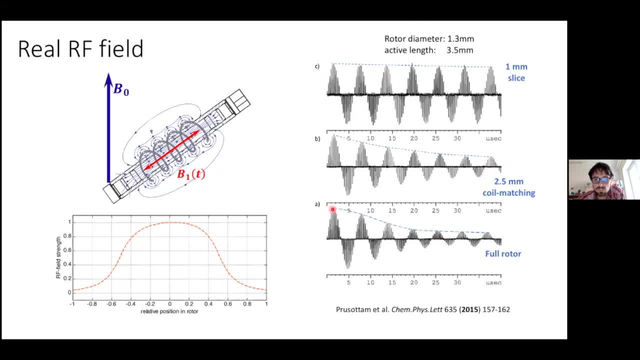 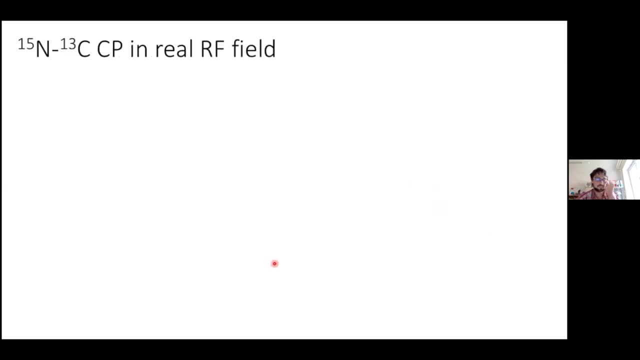 due to this inhomogeneity of the B1 field, the amplitude is decreasing fast, and then you, then you remind only with those things in the middle of the coil. So for the, for the example of the NC CP experiment, which is quite frequently used, 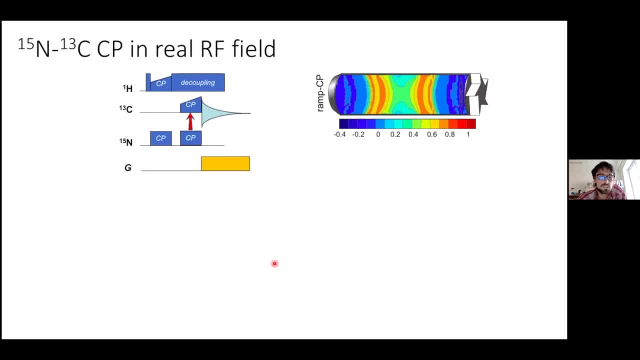 in the protein in the biosolidated NMR. this inhomogeneity of the B1 field actually results in the substantial decrease of efficiency. Here you can see the rotor. This is the NCA simulation of NCA experiment And you can see that there are just few. 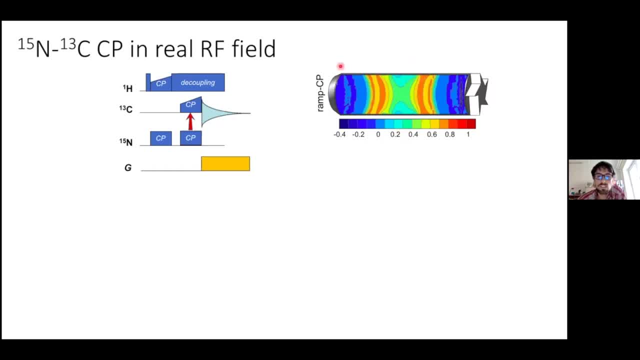 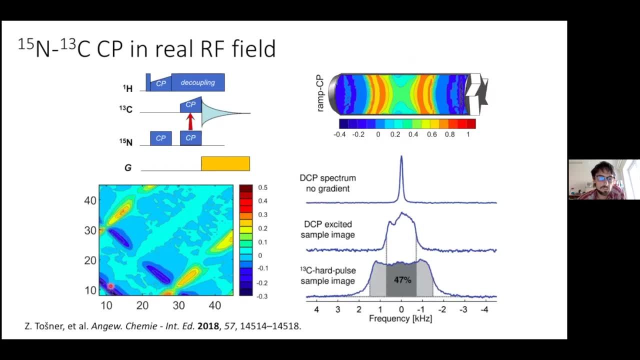 parts of the rotor where you have like reasonable efficiency and the remaining is just less efficient CP. It's caused by quite narrow, by quite narrow Hartmann-Hahn matching conditions which needs to be fulfilled to get correct cross-polarization And in combination with the RF inhomogeneity. 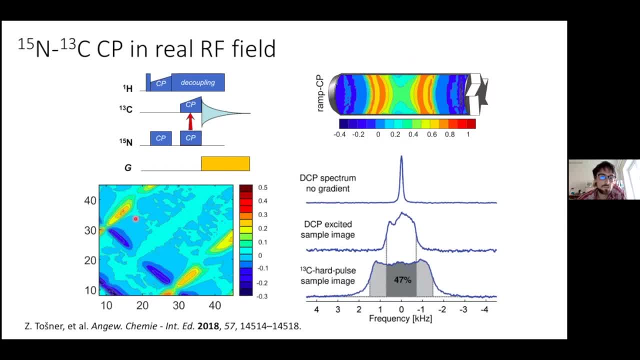 you don't. most of your sample is actually not fulfilling this matching conditions. It can be also illustrated Here where you compare the hard pulse carbon 13 experiment with the gradient applied during acquisition over there And you may see that hard pulse which is more robust. 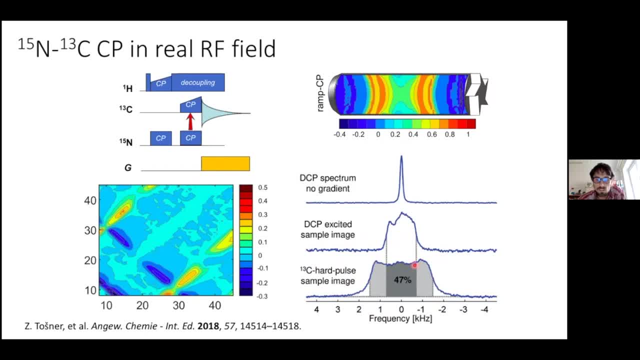 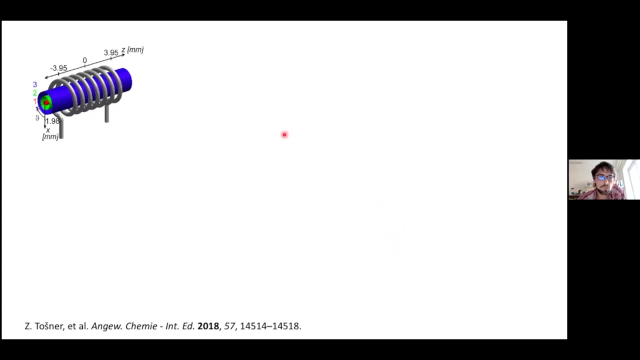 Again, this B1 field- inhomogeneities- gives you by 50% more signal than this DCP, Because because you just select the central part of your sample by the CP element, So we may think about compensating against this inhomogeneities using optimal control. 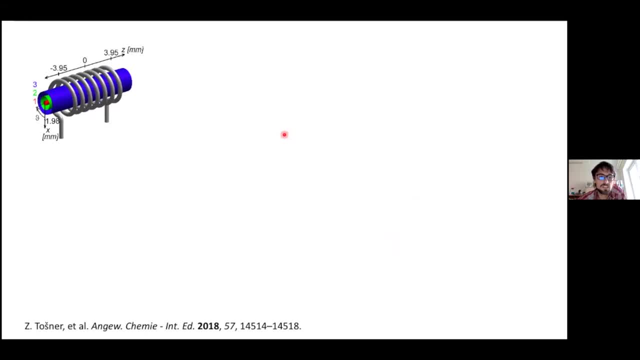 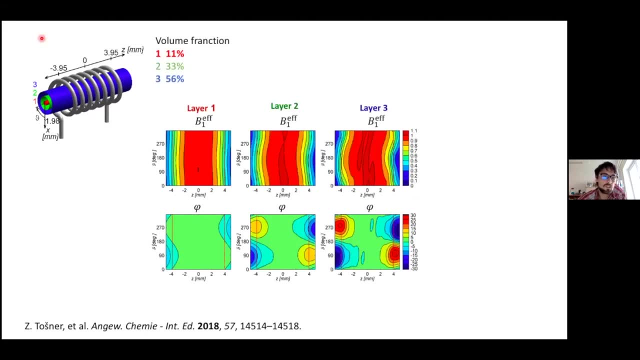 But first we we should have a look a little bit in details how the how this inhomogeneity problems are distributed in the sample. So imagine that your sample actually consists of three layers And for each layer on this plot you can see the variation in the amplitude. 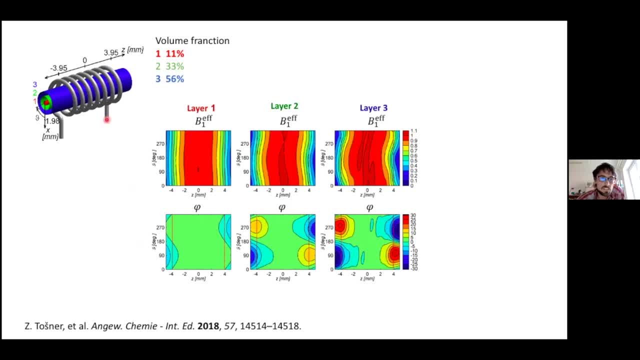 of your B1 field and also in the phase. I should highlight that most of the sample, about almost 60%, is in the outer layer of the sample, when the inhomogeneities are actually the biggest. It's important to remember that. 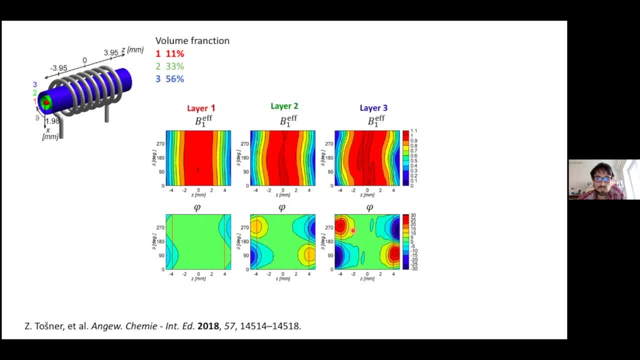 And also I should highlight that the biggest problems are actually not in the amplitude of the B1 field but in the phase of it. So you can see the distortion in the B1 field phase, maybe up to 30%, which is by far not negligible. 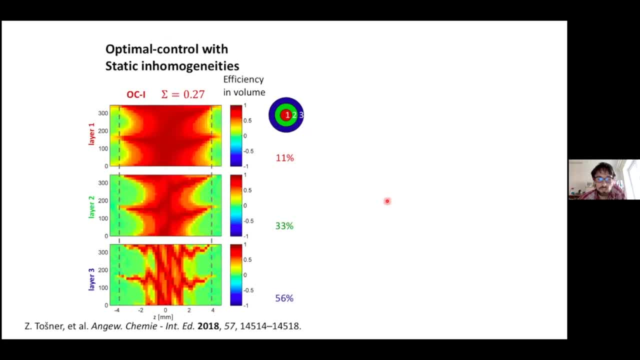 If we try to design optimal, using optimal control, to design the shape which would be, which would be robust and resist this inhomogeneities. you see that on this plot, that we are not too successful. actually, Here is the same, same slices or same cylinders, taken from the 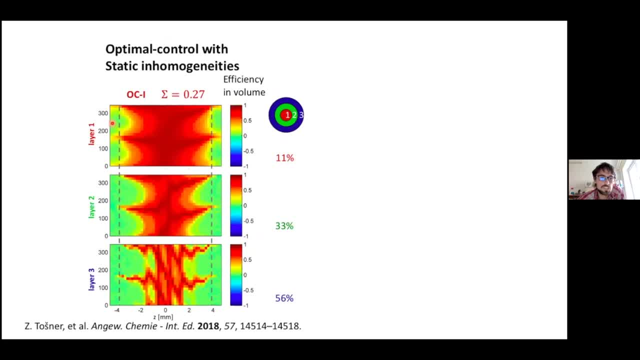 taken from the sample and on the surface of each cylinder. Here you see the efficiency of optimal control, optimal control, CP, compensating just this topic. inhomogeneities of the B1 field And in this outer layer which is, as I said, the biggest part of the biggest portion of the sample, 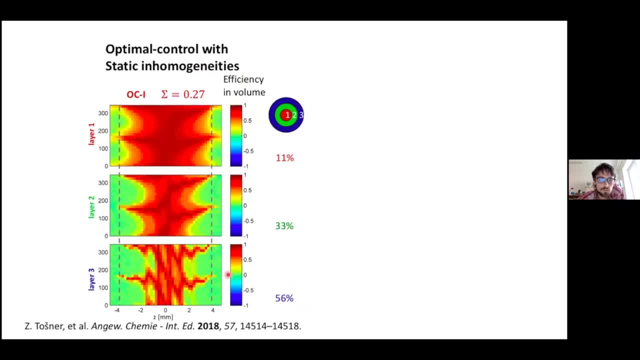 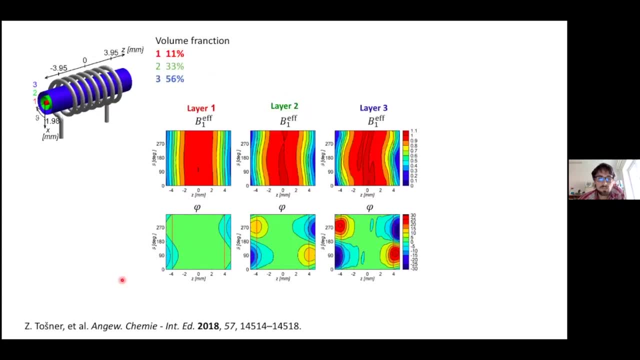 you see that mostly you are around zero efficiency, So it did not work well. but once clever guy comes and realize that sample is actually rotating with the magic angular spinning frequency and it results in the periodic modulation of the phase within the sample, which is now quite complex problem. 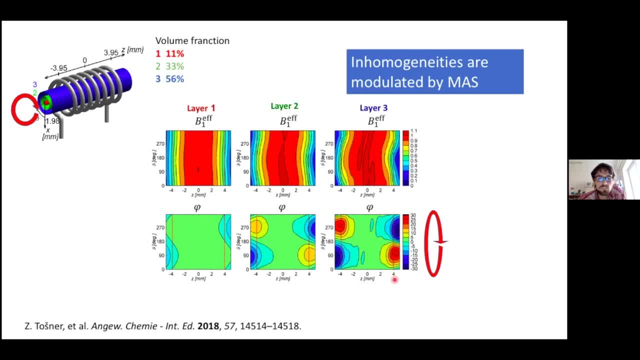 that you have a phase inhomogeneity in the B1 field and in different moment, in different times of the rotor period, the different part of the samples, your different B1 field. but technically this can be also applied in the optimal control algorithm and then we get new shapes. 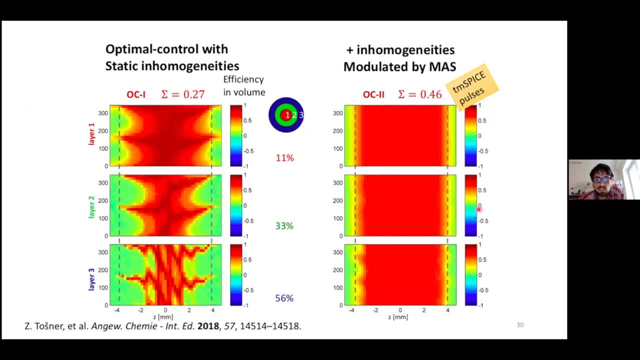 which are now called TM-spice valzists, and they really nicely compensate this, this modulated B1 inhomogeneities, this MAS modulated B1 inhomogeneities, and resulting in the quite nice distribution of the efficient, of the CP efficiency, within the sample. So this TM-spice valzists, 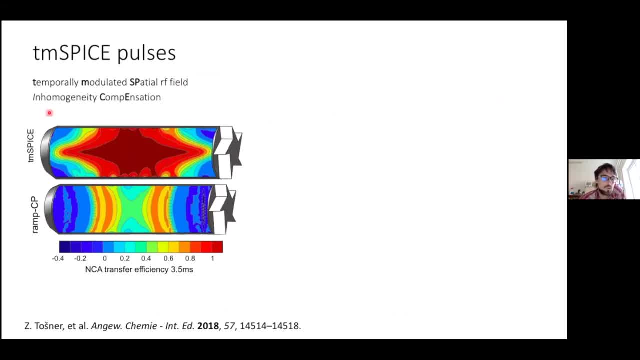 we now look a bit more on the rotor and distribution of our of our CP efficiency. We see that most of the rotor, most of the central part of the rotor, is now actually used in this CP experiment and we observe the signal. Here is the: 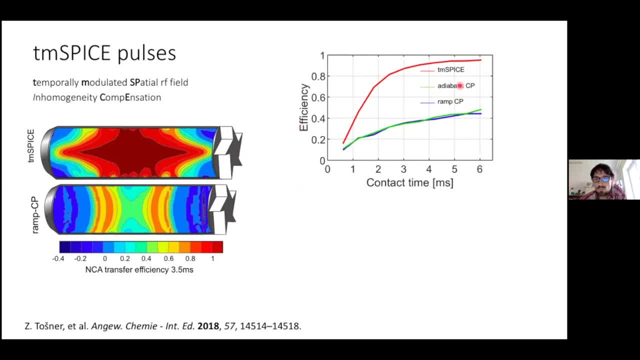 efficiency of the of the RAMP CP, adiabatic CP and this TM-spice experiment And we can see that it's almost theoretically, it's almost two times better than the other normally used experiments. So here is just for illustration how these TM-spice valzists looks like. 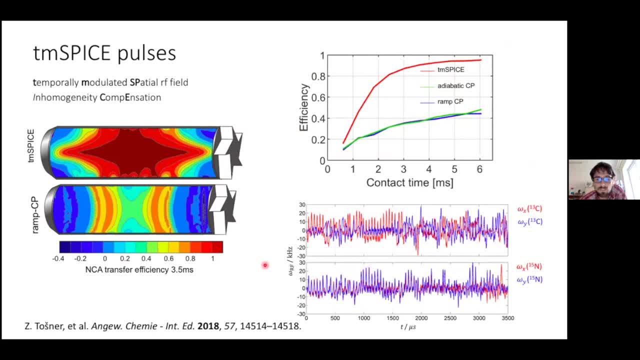 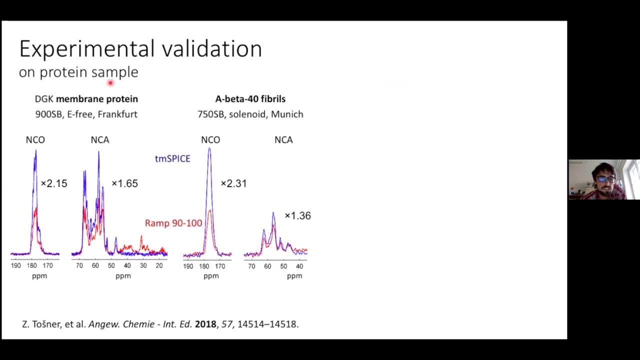 the X and Y channel for both nuclei, And here you can again see some modulation. but it's quite hard to understand how these valzists work. But but we can, we can use them and they are extremely robust. These shapes were tested for several samples and for several transfers, both NCO and NCA, with great efficiency. 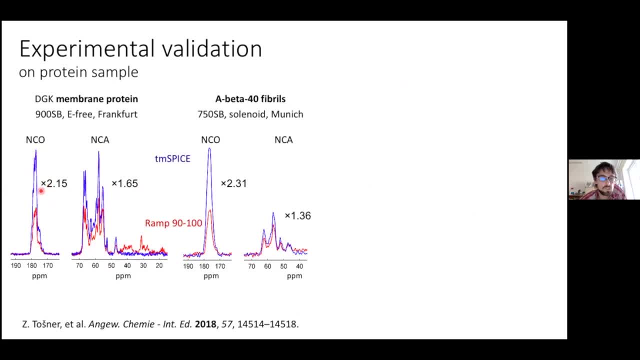 For NCO it's almost two times higher than the, than the well-optimized RAMP CP For NCO- sorry for NCO, it's almost two times higher, And for NCA, where the effects of nearby protons are quite non-negligible. 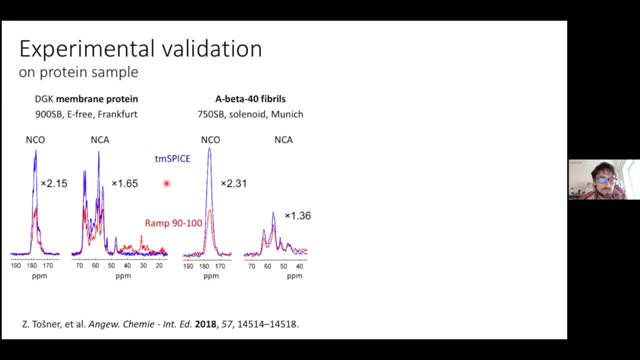 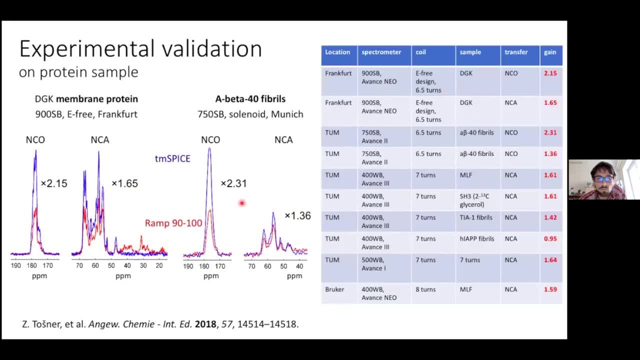 we still gain about about 40 or 70 percent depending on the sample. They were tested on different spectrometers around Europe on different samples, different, different probes, and in all cases we get very nice enhancement and very good efficiency of these TM-spice valzists. 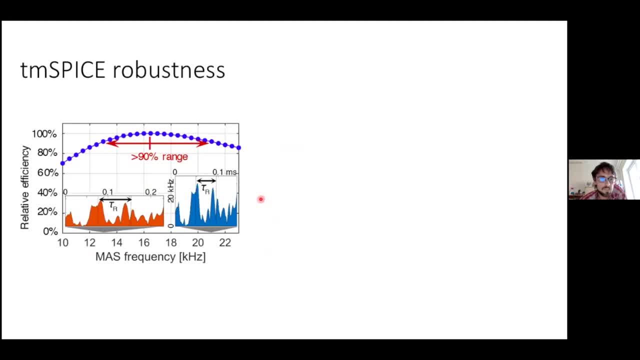 What is great about the application is that they can be also used at a different spinning speed, And only. what only thing which you need to do is actually rescale the length of the pass sequence so that the number of rotor period during the CP contact. 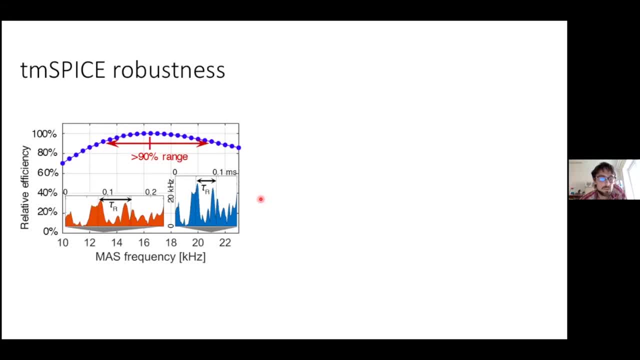 tie is still the same and correspondingly you also. you also must scale the amplitudes, But it works well. For example, in this case we the pass was optimized at 16.5 kilohertz magic angle spinning frequency, but works very nicely from 13 to 21. 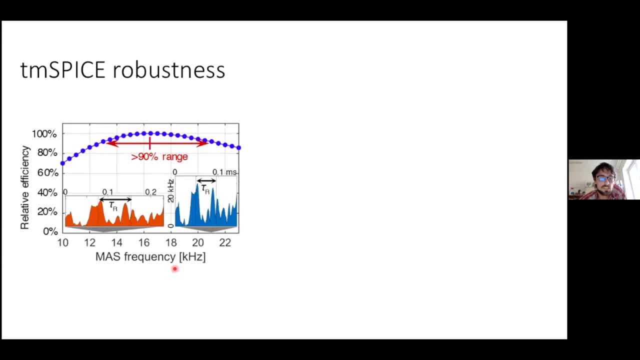 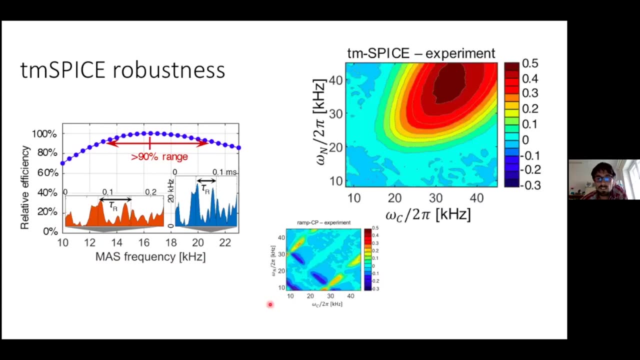 kilohertz, but just with this rescaling and no re-optimization of the shape. So it was the same shape, just just amplitude and length were multiplied by the ratio of magic of mass frequencies. Finally, the big and maybe the biggest advantage of this TM-spice. 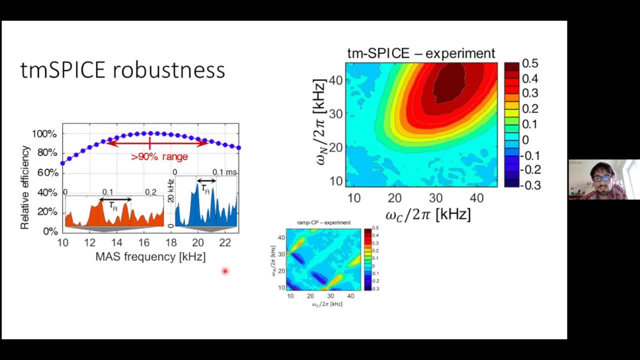 pass is that they are optimized to be extremely robust against RF field homogeneity, which secondary means that they are also robust and works well for different, for different B1 field and does not need to be optimized so carefully in practice. So if you, for example, if you have a look on the RAMP CP. 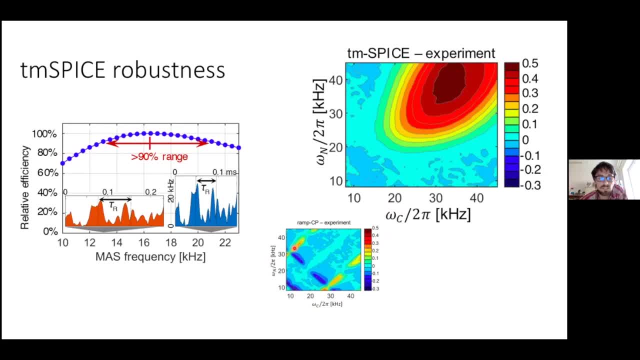 you see that the matching conditions are quite narrow and to get maximum signal you must quite carefully find the hotspot of your magnetization transfer. For the TM-spice, you just roughly estimate the using pulse calibration. You just roughly estimate the correct amplitudes of the 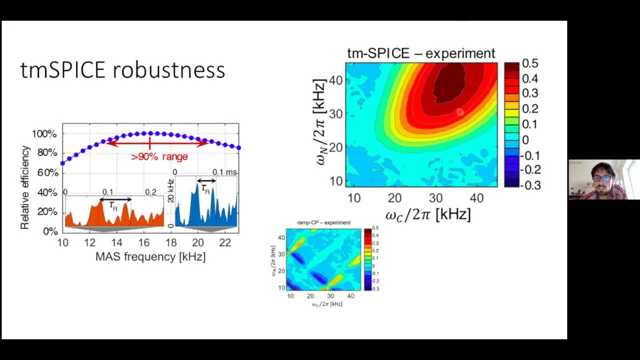 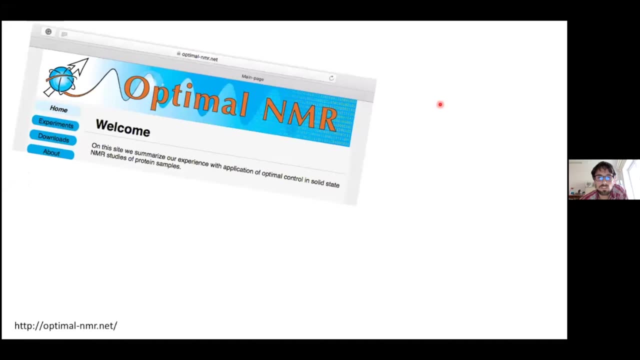 of the RF passes in both channels and get this big hotspot of the efficiency, which is great, And it's actually hard to miss this point when you are using TM-spice passes, TM-spice passes. So that's it. And there is one more practical thing about TM-spice passes, and it's that. 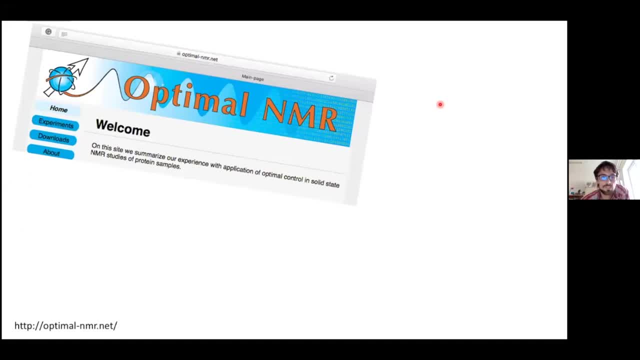 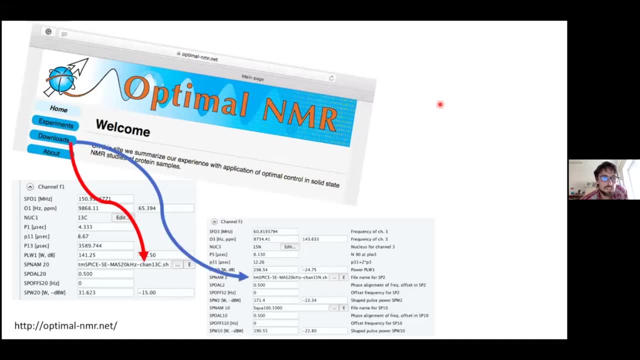 many of them. you can now download from the web page of Zdeněk Toszner Group this optimal NMRnet. You just download them. put the put the download shape to your to your spectrometer control computer. You should correctly calculate the length of the pass sequence. 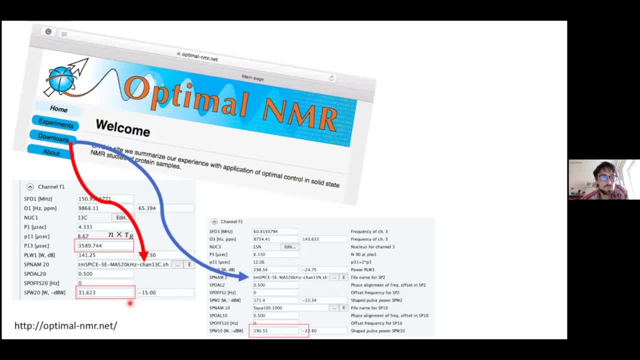 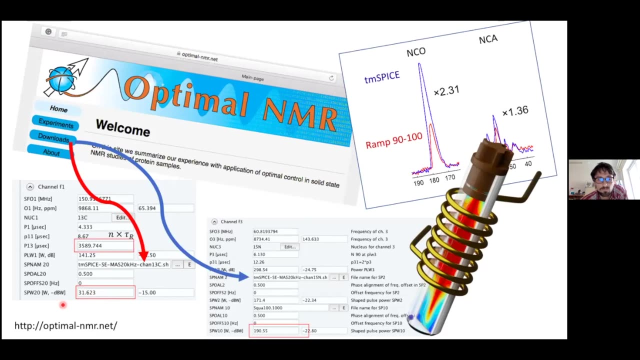 You should correctly calculate the power to to correspond to what's what's actually written in the in the headings of this pass. And then you get nice B1 field in homogenic compensation and also great NCO or NCA transfer. So that's all from my side about optimal control. 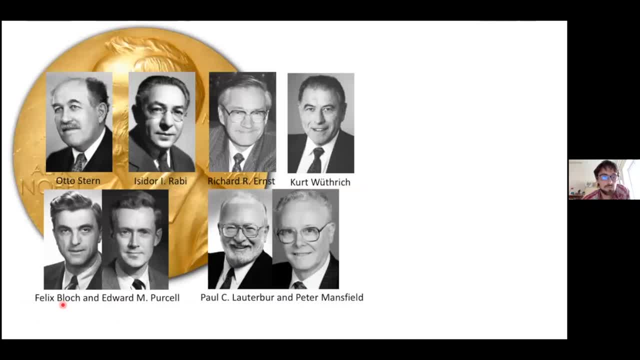 And in this point, as every talk about NMR should show these guys having Nobel Prize, I suggest you at one point one more guy, which is Leonid Kantorowicz, who actually get the Nobel Prize for economy, for using optimal control theory. 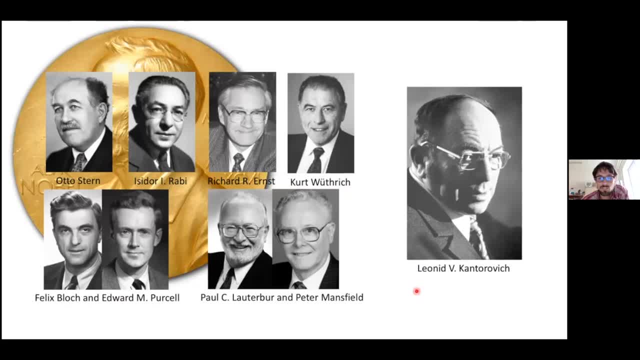 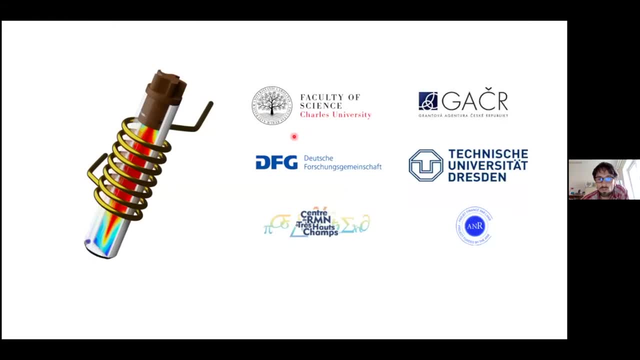 So we have one more Nobel Prize in the in the field of NMR. Finally, very much thanks to especially Zdeněk Toszner and also all my friends and collaborators from Lyon, from Dresden and also from Prague. OK, that's all from the second part. 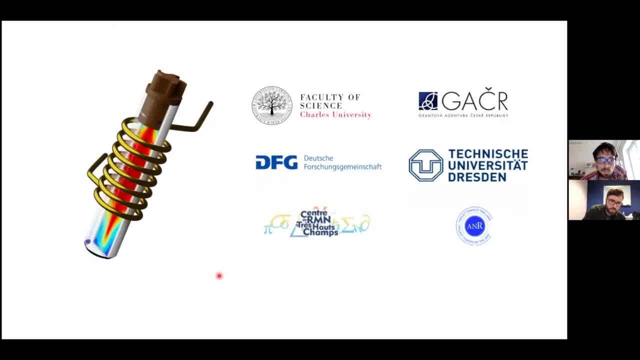 All right. Thank you very much, Jan. It's a very nice talk. We already have a few questions. Feel free to continue to add them in. I know that we're approaching the end of the hour, So thank you everyone who has joined us for the discussion of optimal control today. 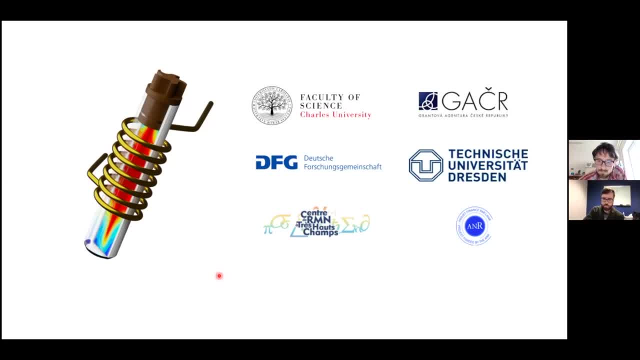 And feel free to come back and join us in two weeks time. In the meantime, let's get to these questions. So we have one from Ilya Kuprov saying the solution is an ill-posed operation in the Hadamard sense, so not unique, not stable. 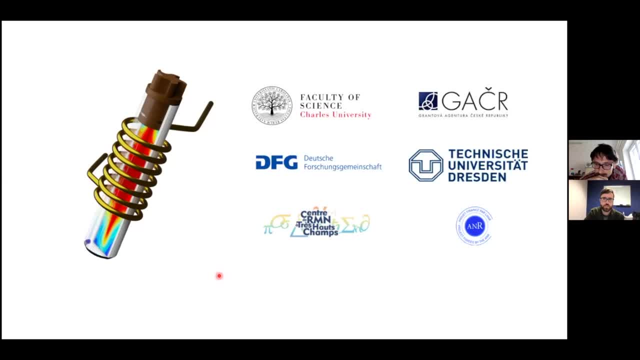 So how do you actually obtain the pulse shape that would then yield the desired shape at the sample? Ooh, I think we don't need it, because we- I think I have- I have tried to show you that this, these things, are quite robust against that. 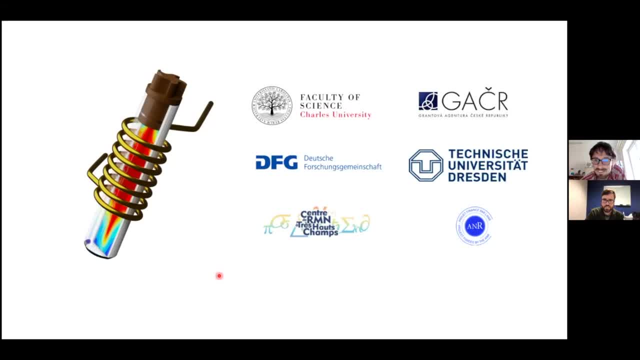 So, but maybe this should be discussed like more in details. I would maybe need to get this question more clarified. Ilya also adds: just to add: congratulations on cracking this homogeneity problem. We're suffering from that a lot in ourselves. 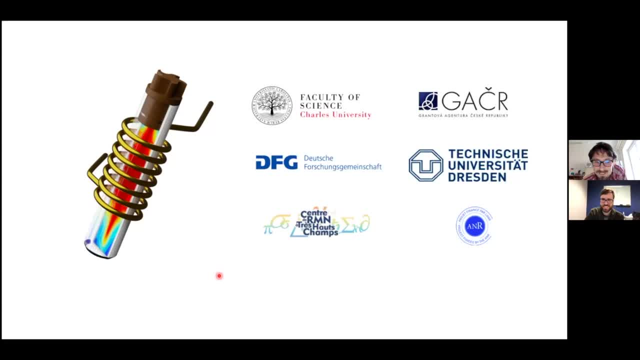 It's mostly congratulations to Zdeněk Pošner. I have just presented that. but it's great. Yes, Thank you. Thank you very much. Then we have a question from Moreno saying: did you test the TM spice at MAS of 60 kilohertz and above? 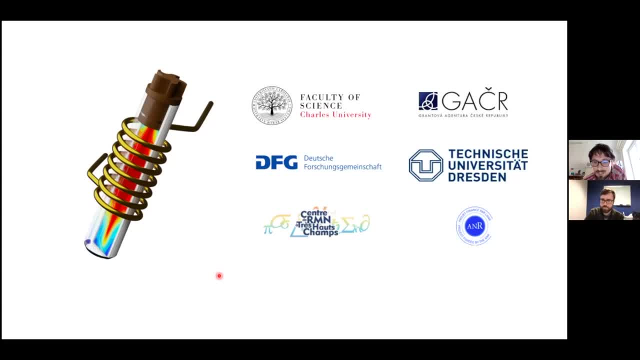 Yes, Yes, I have personally tested them in Lyon for different samples and they work quite well for 60 kilohertz And also I did a few tests and 100 kilohertz and it works. It works, So sometimes it's- it's not like factor of two- better than RAM. 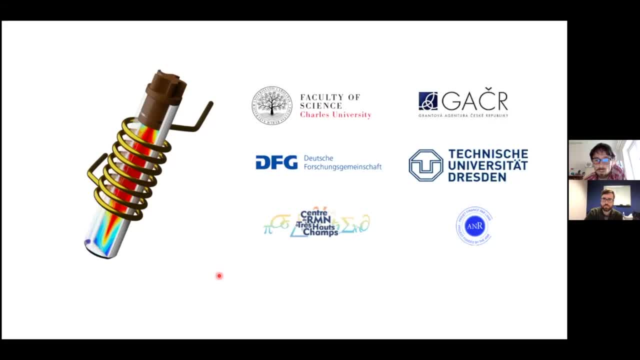 but in all cases it means that I spent a lot of time to correctly optimize the RAM for the maximum efficiency and then I just put the, put the TM spice there, having like the calculated value of power, and it works at least the same. So so sometimes it's not such a big gain. 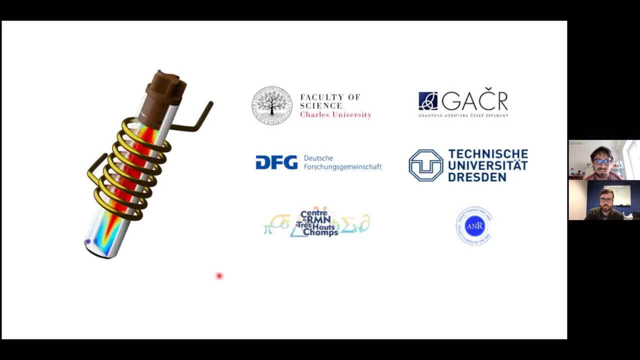 in absolute numbers, but the gain in time is great and in the comfort of users. So it works also at fast MAS. But one should be probably careful with the scaling up of these shapes, So if you need to use them at 60, it would be great to have some which are: 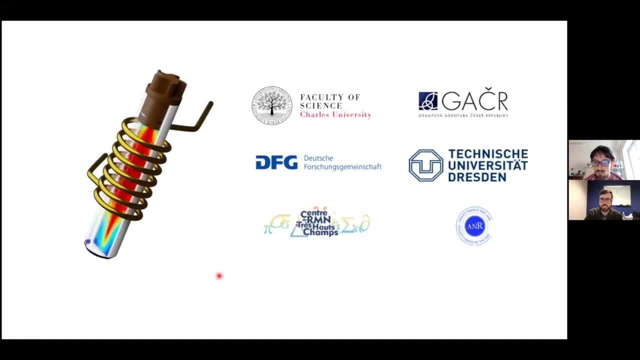 optimized close to 60 kilohertz, not those at 16.5.. But feel free to ask for anything that you need and you don't find it on the web page. And we have a question here from Nassif asking: in the TM spice schemes are modulations in the RF pulse amplitude? 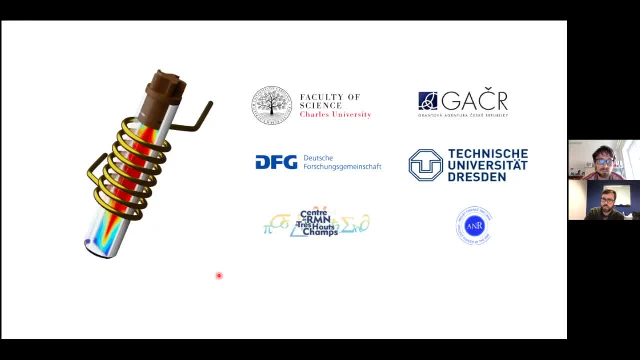 rotor synchronized or are they not Usually? if you have a look on the shape, sometimes it looks that there is some rotor synchronized modulation, but it's not always And it's usually a feature, but not for both, sometimes not for both channels, maybe not for. 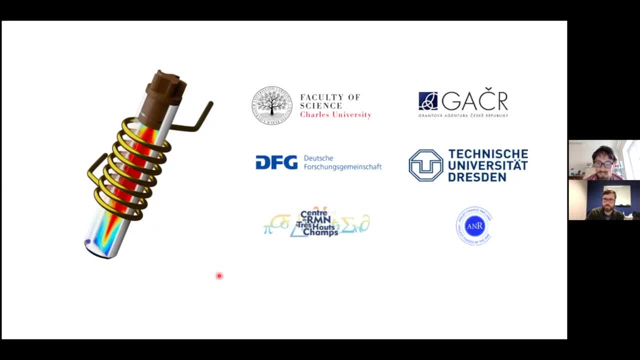 all moments of the pulse. So this feature is there, it's present, but it's not general. So we we can't easily take, for example, just one rotor period and repeatedly apply it over the time, But modulation is by spinning. speed is quite evident. 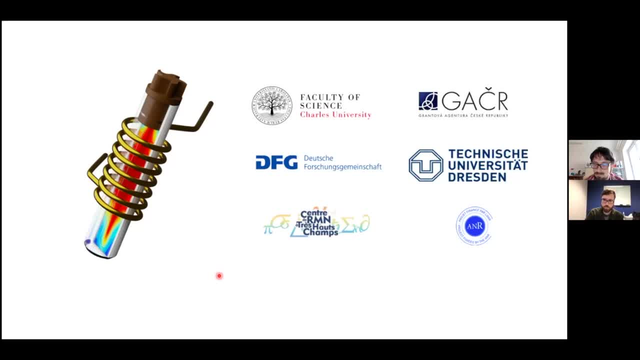 Nassif has a follow up question. can RF inhomogeneity modulation affect under MAS be compensated for any pulse speed scheme as well? So, if I do understand correctly, the question is about inhomogeneity and 100 kilohertz. MAS Didn't specify a number, but just the RF inhomogeneity modulation. 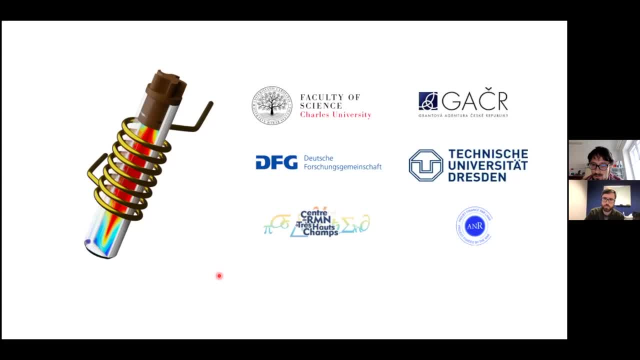 under MAS be compensated for any pulse speed Principally, yes, yes. So some of the path, We found that some of the paths, some of the schemes are more robust against RF inhomogeneities Typically, for example, redor is quite robust. 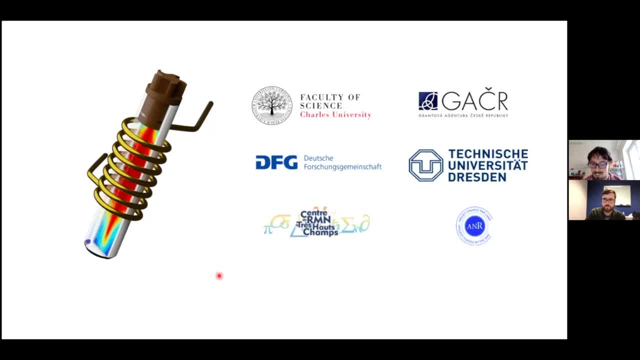 This XY8 phase cycle is kind of magic. I think the guys who found it probably have know what they are doing, but it's great. So, but there is probably plenty of sequences where it could help- quadrupolar nuclei and others, Yes. 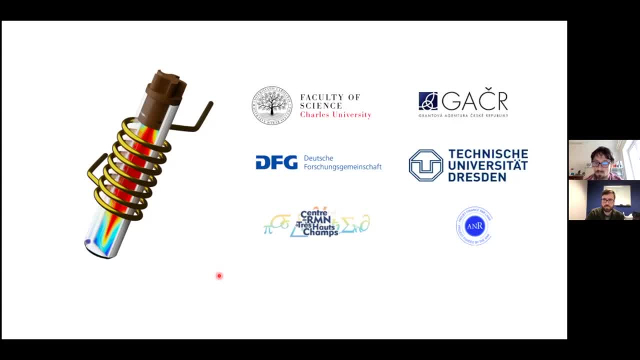 So in principle can be Yes. And Dominique Maceo has a question on: is your approach sensitive to the pitch of the rotor? Do you mean to the correct angle Of all of the? so it It was not tested, I think, and at least I'm not aware of that. if it was tested, 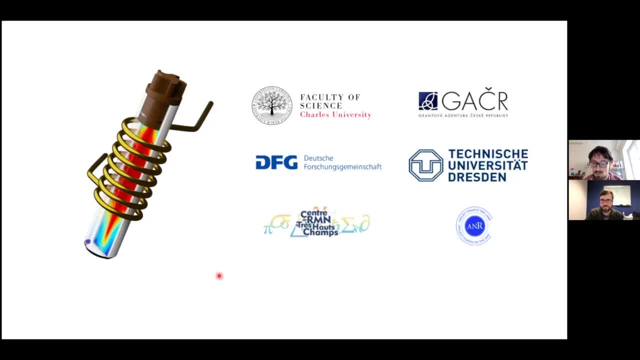 But technically it can be another parameter to make the sequence robust. Yes, but this was not tested. Sorry, I don't, I don't know. I hope it's not And I hope everybody of you have a correct magic angle. All right, And then we have an anonymous attendee. 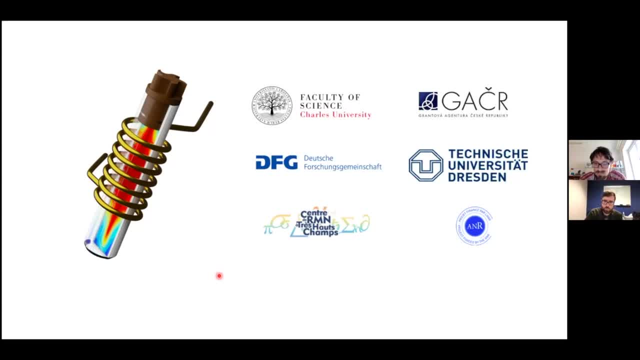 who asked or mentioned amazing enhancement. You mentioned that one age contribution is making the NCA And it's lower. You comment on the possible application of HN or HCCP And Eric Yuan kind of responded to that, saying the transfer in general but no CP. 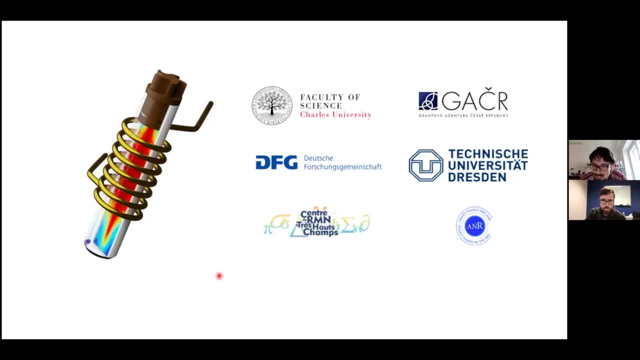 Can you? can you read it again? I'm not sure if he's asking about decoupling or something else. Don't mention that the one age contribution is making the NCA enhancement lower. And then you comment on the possible application to HN or HCCP. 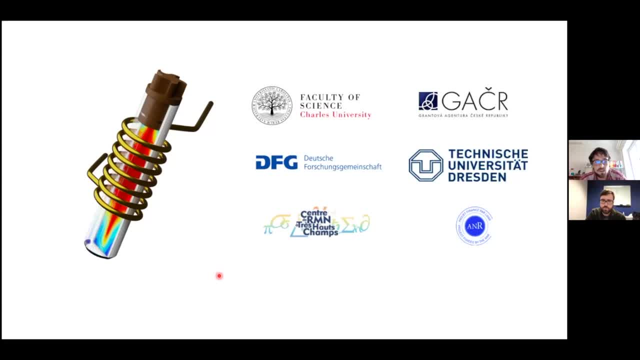 I see, I see, OK, OK, So. so application in HN and H HCCP. maybe it was tested. Apparently, the- this is the coupling between proton and carbon, or proton or nitrogen- is stronger, the improvement is not such a big. 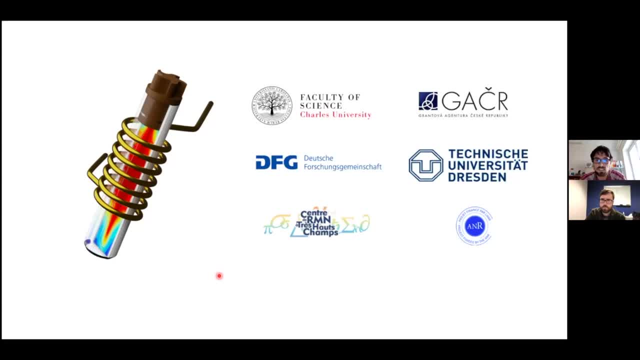 There will be still this, this nice effect of the, of the easy optimization, And we don't have such a factor of one point five improvement in H and HC, probably just because of stronger coupling, But in principle it could work. I maybe should should highlight here what is quite important is that for an age 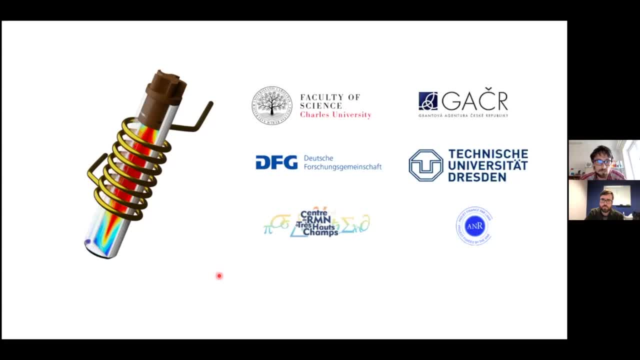 transfer, and see transfer actually. So we always put on the proton decoupling to to reduce the effect of the nearby protons Which are, which are bad actually and how hard to model correctly. so so, But the answer is, it also works for HN, but with not so efficiently. 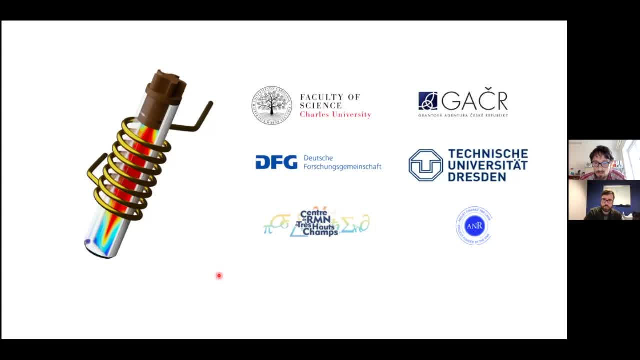 Then Marina has another question saying: did you need special decoupling on one age during NCA with the teams Spice or CW decoupling? We use CW and it works well. I mean, it works, it works. And he also mentions, by the way, very nice.